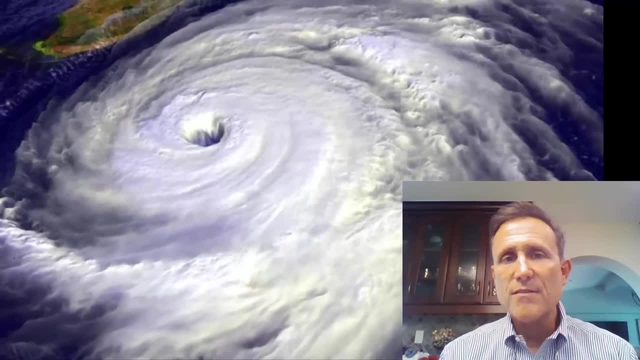 Welcome to Introduction to Meteorology. I'm your instructor, Dave Cacciarella, and in this course we are going to take a look at atmospheric sciences, of course, weather and weather phenomena and weather forecasting. It's going to be a great course. You're going to have the opportunity to view these lectures covering each chapter of the textbook. 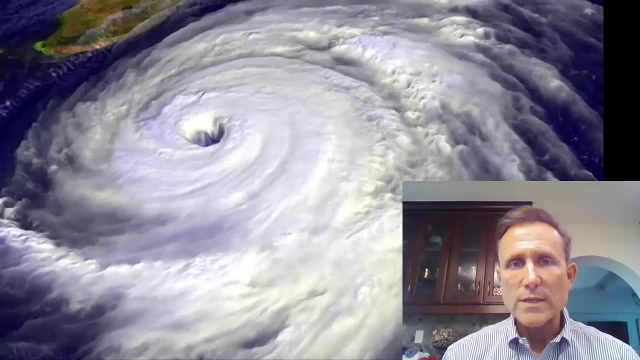 There'll be additional podcasts drilling down on some of the more important topics and other course materials that you can use to learn all about well: meteorology, atmospheric sciences, weather and weather forecasting. But first we're going to start out with a little bit on the history of meteorology. 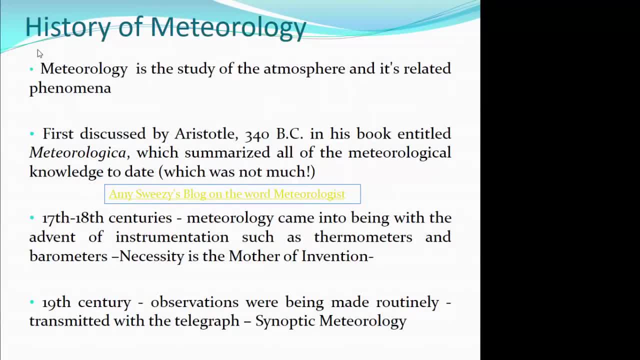 The history of meteorology. Well, we'll start there Fairly brief. meteorology is the study of the atmosphere and its related phenomena. It was first discussed, believe it or not, by Aristotle way back in 340 BC in his book entitled Meteorologica, which summarized all of the meteorological knowledge to date, which at that time wasn't a whole lot. 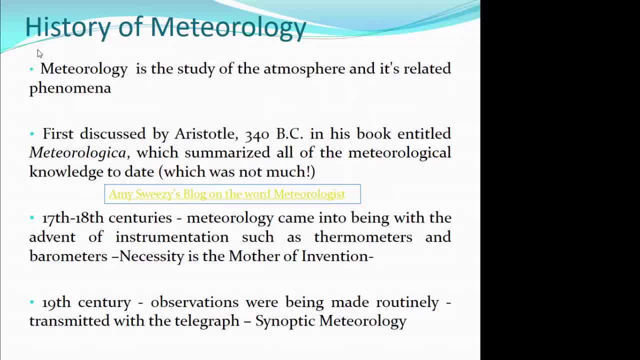 In the 17th and 18th century, the development of meteorology was a function of necessity. is the mother of invention, And what was the necessity? Well, traders at that time trading goods by ship were losing cargoes and vast amounts of money because of the loss of those cargoes due to the weather. 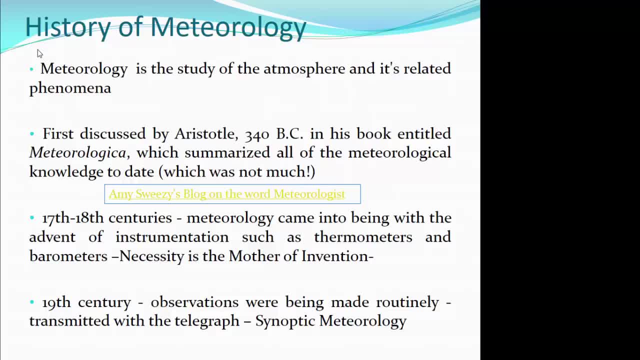 And those wealthy traders wanted some way to figure out what the weather was going to be like, so their ship captains would know which way to sail. And so necessity be the mother of invention. Well, the invention was the barometer, And a barometer was nothing more than an instrument that measured atmospheric pressure. 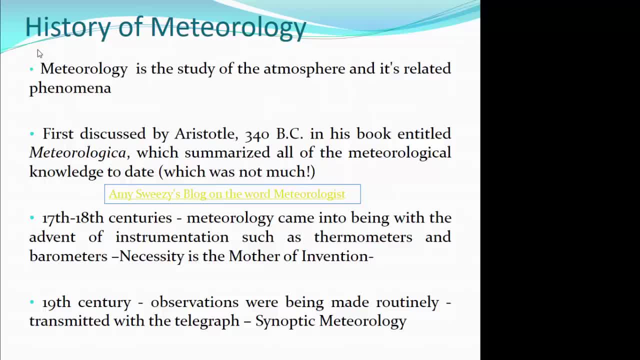 Was the pressure rising or was it falling? And what we knew at the time was: rising pressure meant fair weather- sail in that direction. and falling pressure meant foul weather- sail away. So the first barometer back in the 17th century helped ship captains. 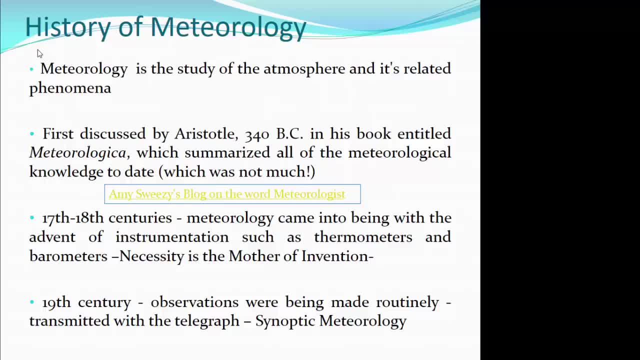 save their cargo from bad weather. In the 19th century, observations were being made routinely And they were being transmitted by telegraph. So somebody, let's say, in Spain, could transmit the observation of their weather to somebody in England or France. 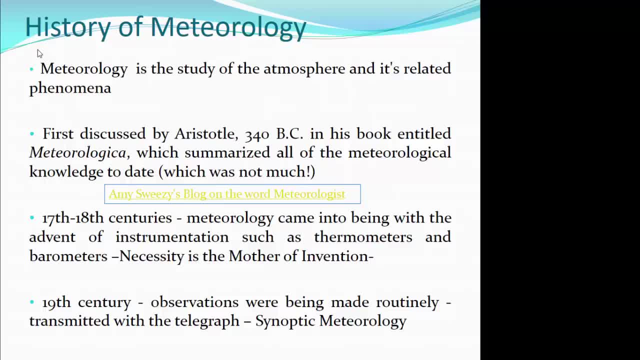 And because we knew what was happening in different parts of the continent, we had the development of synoptic meteorology, Synoptic meaning. at the same time, People in different parts of a large geographic area knew what was happening with the meteorology. 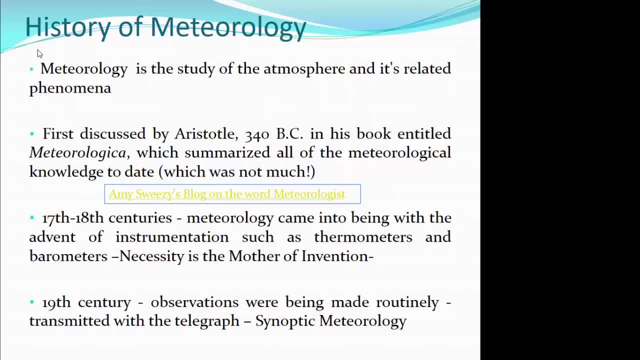 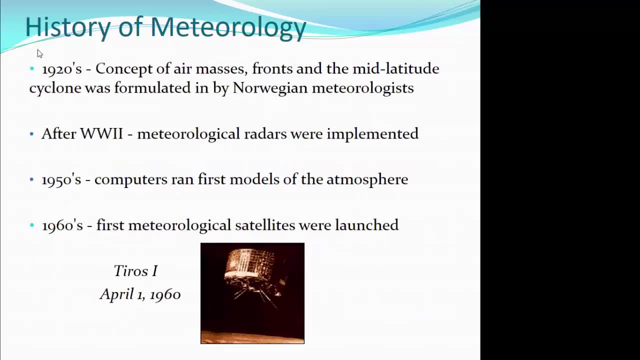 With the weather at the same time, And that was the advent of synoptic meteorology. In the 1920s, the concept of air masses, fronts and the mid-latitude cyclone was formulated by Norwegian meteorologists. The Norwegians were big into weather. 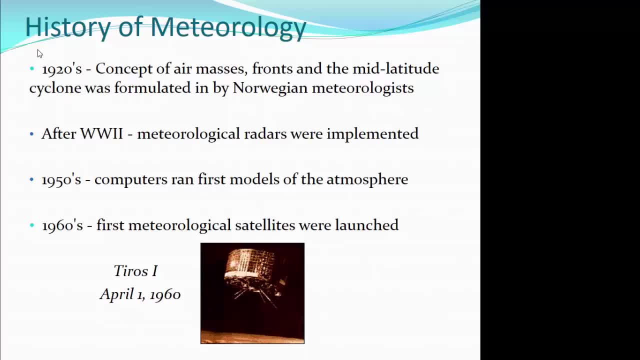 And what they came up with was the concept of air mass, And what separated air masses were fronts, And as air masses moved along, mid-latitude cyclones formed, And we're going to talk an awful lot about mid-latitude cyclones. 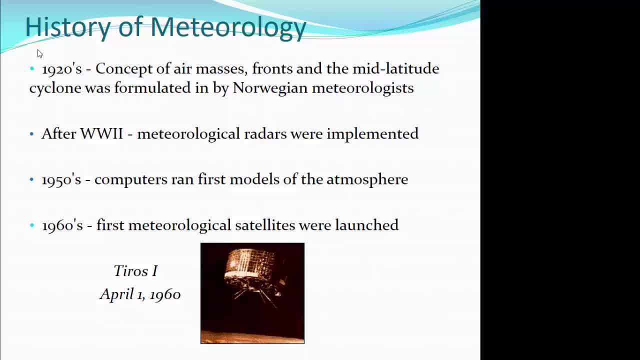 And what they mean to our weather each and every day After World War II. well, military leaders began to realize, and they always did, But they really had the sense of how important weather was after the D-Day invasion And which was hampered and delayed by weather. 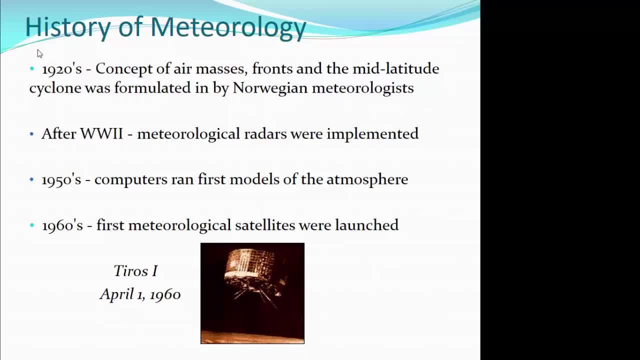 So, the US military being the most powerful force on the globe, they decided they wanted to know more about the weather than anyone else, And they had some mathematicians, And those mathematicians sort of said, hey, you know what? 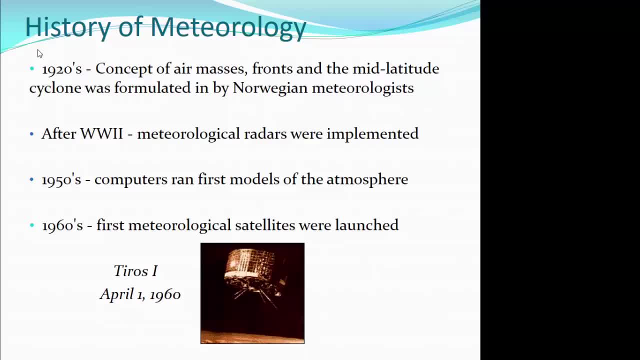 We have these calculus equations, These very advanced mathematical equations that can predict what the weather is going to be like in the future. But these mathematical equations take longer to solve than the time that they predict, So you solve them after the time has already occurred. 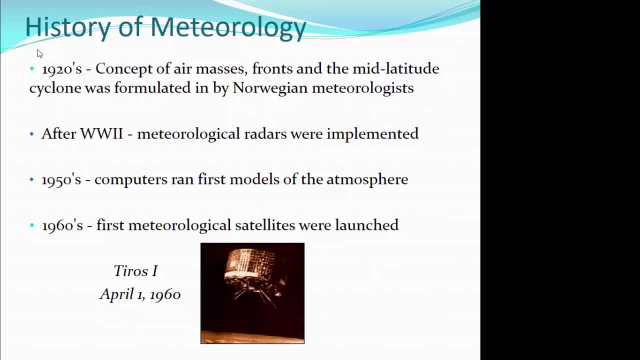 Doesn't do you a whole lot of good? Military leaders thought, well, if we could do the computations faster, we could have an actual weather model that predicted the weather. So they needed a faster computing machine. The faster computing machine Came in the 1950s from IBM with the first computer, UNIVAC. 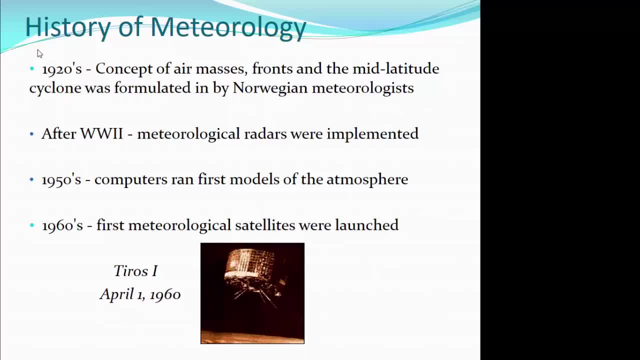 So the very first computer was developed and built for the US military to solve weather models. That's why you have the smartphones in your hands now. In the 1960s the first meteorological satellites were launched- Trios 1.. 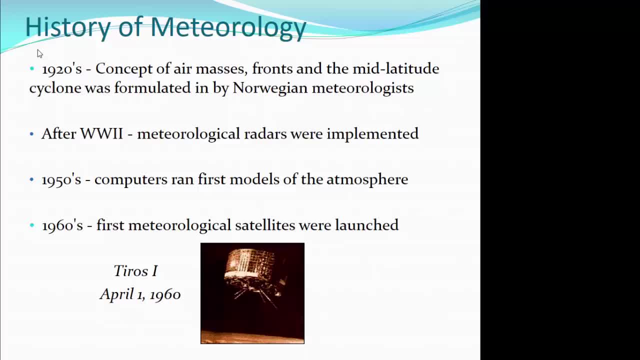 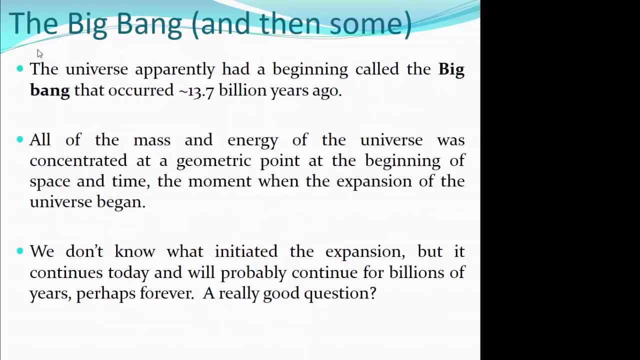 That was April 1, 1960. Ushering in a whole new era of synoptic meteorology. So to understand the weather, we have to understand the atmosphere. To understand the atmosphere, we have to understand the formation of the planet. 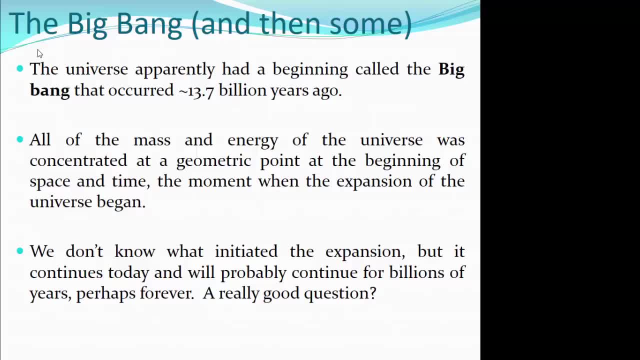 For that we have to understand the formation of the solar system And for that, ultimately, the formation of the universe. Now, these different factors that we'll be discussing on this particular slide have to do with significant scientific theories that are largely accepted by the vast majority of scientists. 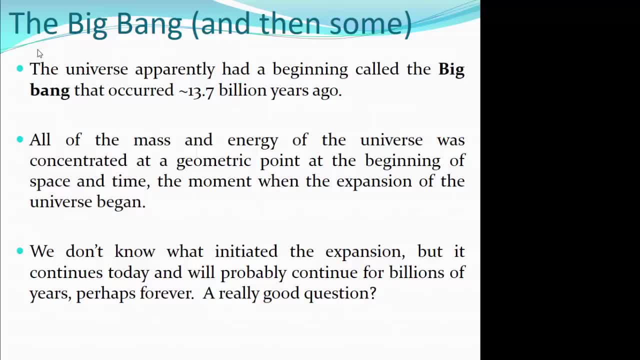 They may actually come into conflict with some of the world's most important scientific theories. They may actually come into conflict with some of the world's great faiths, But these are scientific theories that are currently accepted by the scientific community. If it conflicts with your particular faith, please understand these are theories. 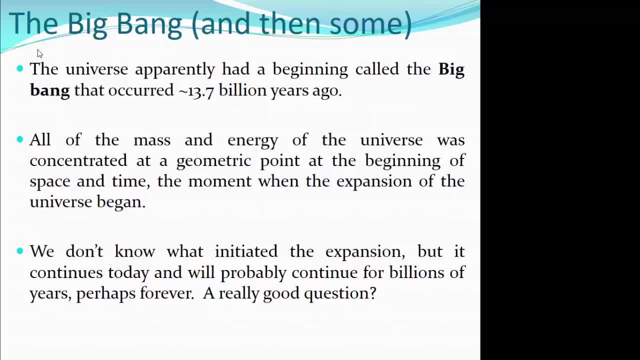 You will not be necessarily tested on these subjects, But just to give you an idea of the general scientifically accepted formation of the universe and solar system. And the universe apparently had its beginning with the Big Bang that occurred about 13.7 billion years ago. 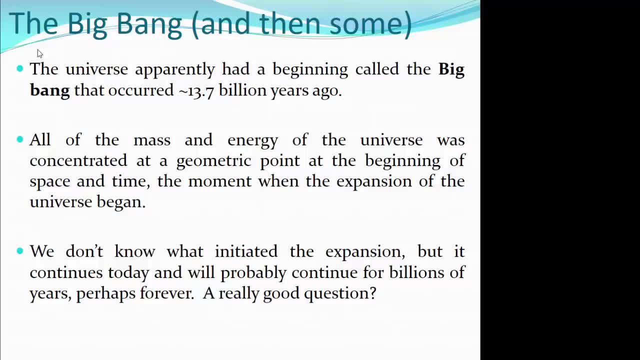 All of the mass and energy of the universe Prior to the Big Bang was concentrated at a geometric point in space and in time, And that was the beginning. And when the expansion began, it was a violent, explosive expansion And the universe began to expand outward. 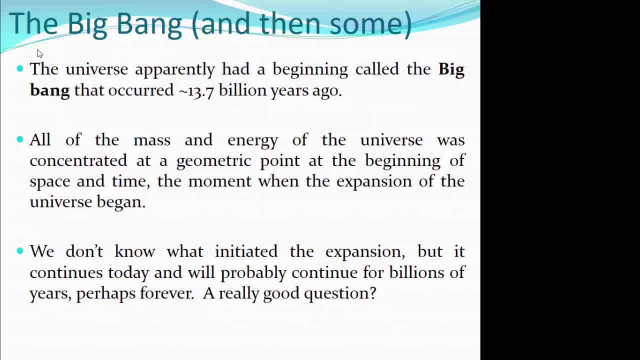 And continues to do so at this time. We don't know what initiated the expansion, But it does continue today And probably will for billions of years. So a really good question: Will it go on forever? Will it continue to expand? Will it expand to a certain point and then begin to contract? 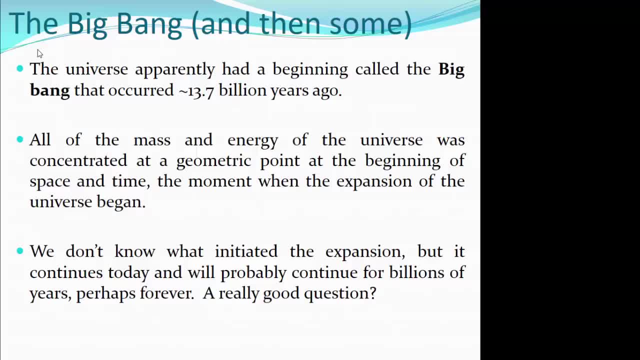 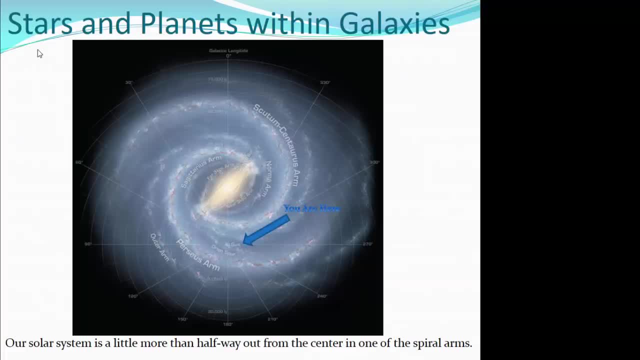 Or will it expand to a certain point and then just sort of flatten out and become static? Once the Big Bang had occurred, all of the elements of the universe were rushing away from one another, as the universe expanded Very hot and very rapidly After several million or maybe even hundreds of millions of years. 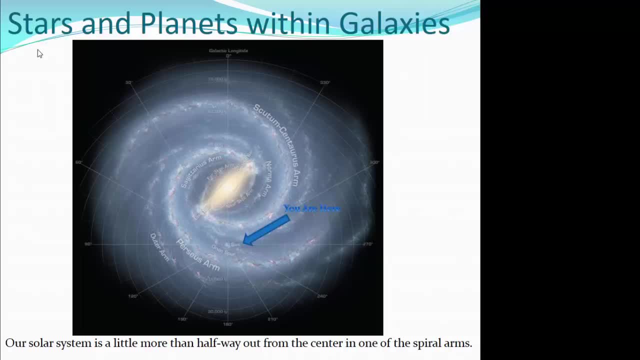 The universe began to cool, Condensation into galaxies and solar systems and suns and planets began, And those galaxies containing solar systems, suns and planets were interspersed all across the universe, Our galaxy, the Milky Way, And here's a map. 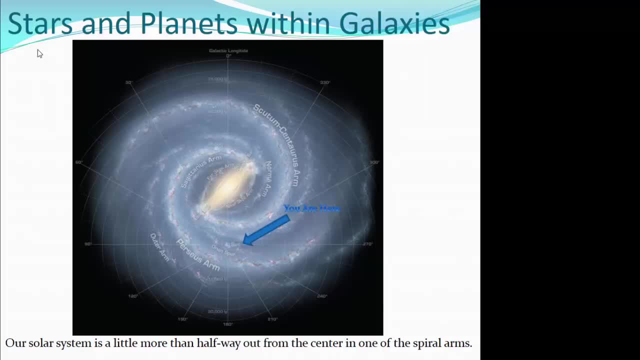 The very center of the galaxy, that galactic core. That's not one big, gigantic star, That's just where all the stars are so tightly packed together It looks like one big star. The sun is a little more than halfway out from the center of the Orion Spur. 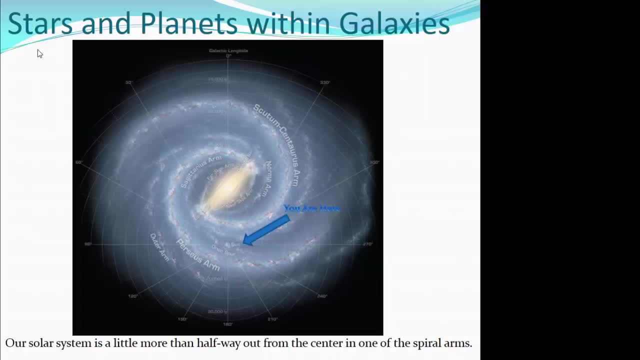 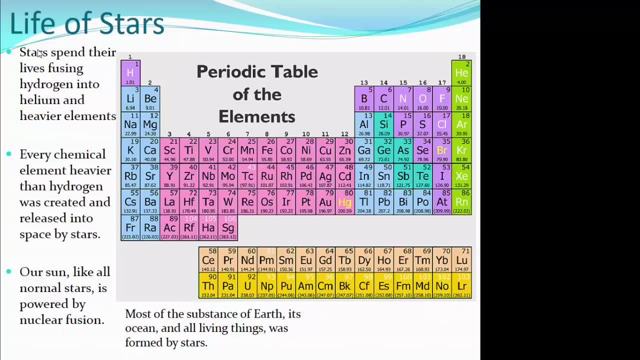 One of the spiral arms. That's where you can find our solar system. What kind of a life does a star have? Well, a star spends its time fusing hydrogen atoms into helium atoms And then, eventually, the hydrogen and helium being fused together to make heavier elements such as lithium, beryllium and boron. 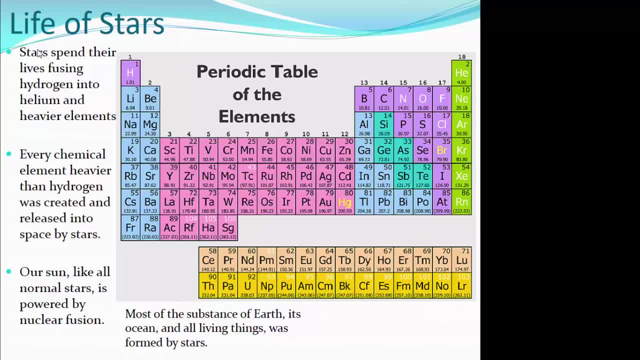 Once you get much higher than carbon. Though they're too heavy the atoms, to be forced together by just the powerful nuclear forces of the sun, It takes a much more powerful force, The explosion of a supernova, And that typically happens in larger stars. 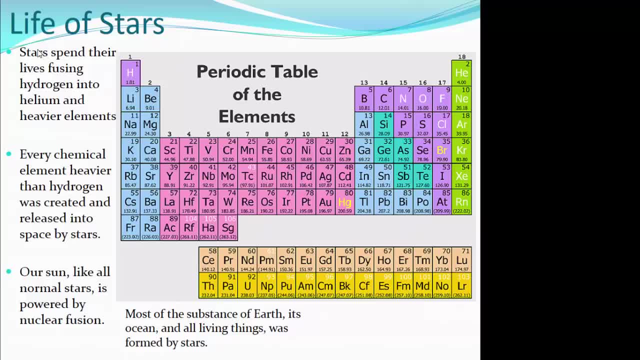 So what happens in a star? Every chemical element heavier than hydrogen was created and released into space by stars. Stars are massive, massive things, And the weight of all that mass creates tremendous gravity. That gravity creates gravitational friction and heat. So now you have both pressure from gravity and heat. 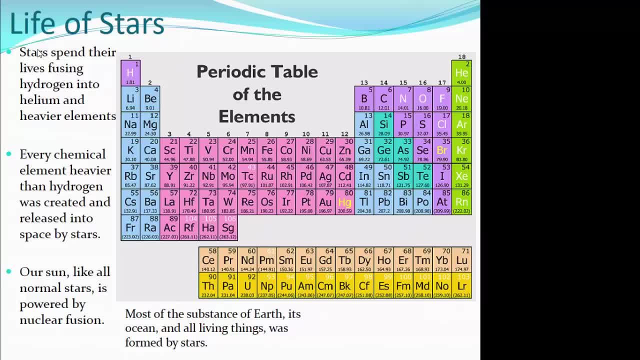 And enough pressure and heat forces atoms together. In this case it's the atoms of hydrogen. If you take four hydrogen atoms and you force them together, they become helium. Well, you can see from the periodic table that the hydrogen atom weighs 1.01 atomic units. 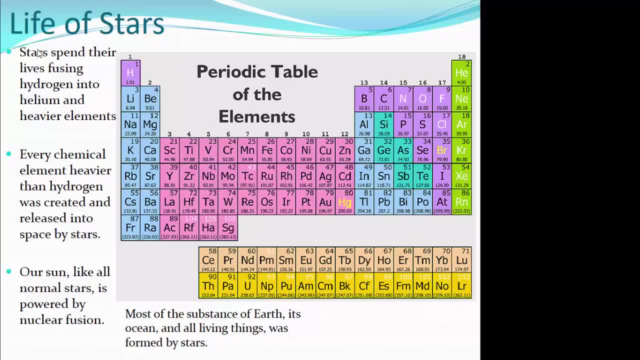 While the helium atom weighs 4.0 atomic units, Four hydrogen. Hydrogen, then, should equal 4.04, to make it a helium, But it only equals four. So what happened to that .04, that atomic mass? Well, that is what is converted into energy. 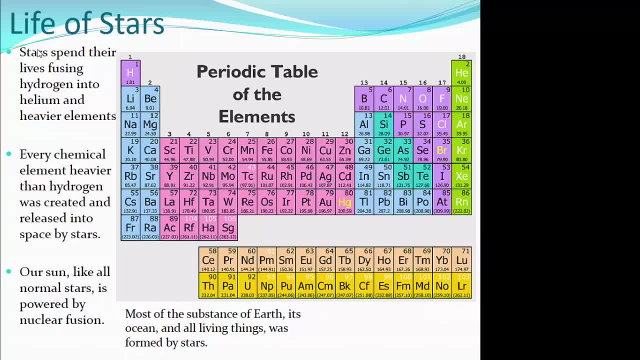 And is the radiation or the energy of the sun. So our sun, like all normal stars, is powered by that nuclear fusion. As the sun continues to use up its hydrogen, it begins to force helium together with some hydrogen to get the lithiums. 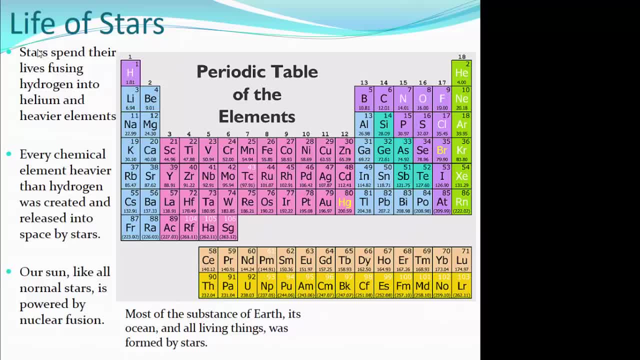 And as it uses up the helium and the lithium, it begins to force things together to become the beryllium, And again We can't get much higher than the carbon. When suns explode, large suns- the supernova forces all those other elements together, creating all the other elements of the universe. 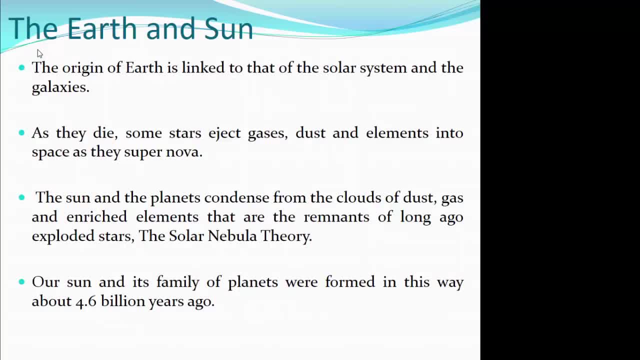 The origin of the earth is therefore linked to that of the sun and the solar system and the galaxies. As some stars die- large stars, they supernova and eject that gas and dust and other elements into space. That gas and dust and other elements eventually, as it cools, will condense into new suns and solar systems and planets. 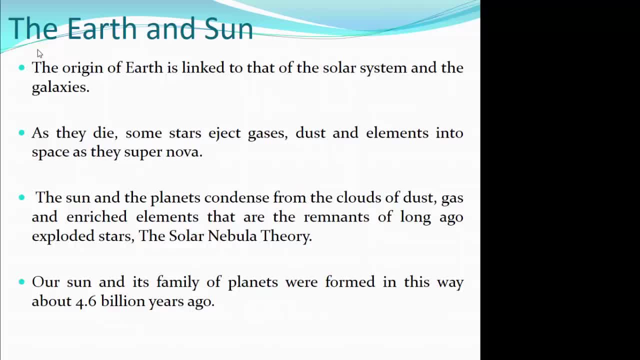 And that is known as the solar nebula theory. The sun and the planets condense from clouds of dust, gas and enriched elements that are the remnants of long ago exploded stars. Our sun is thought to have- is theorized to have- formed through the solar nebula theory about 4.6 billion years ago. 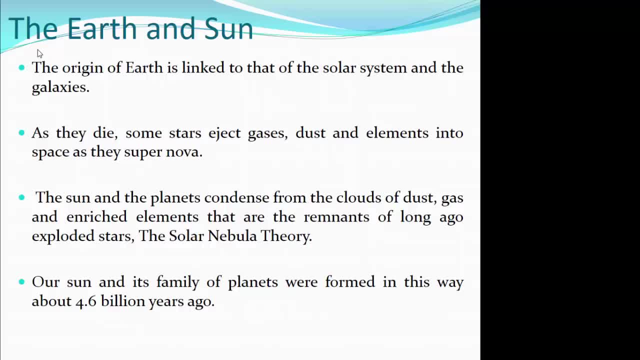 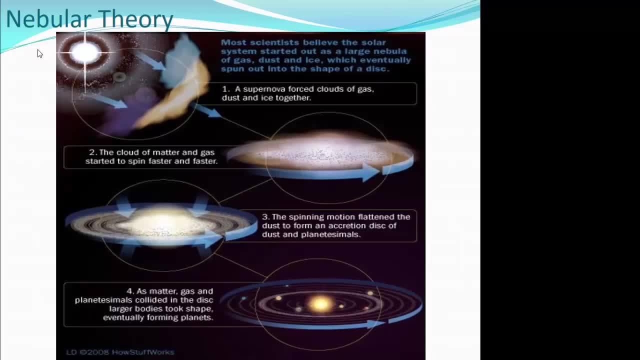 And as the sun formed, so did the planets, at generally the same time or shortly thereafter. So here is the solar nebula theory, Sort of played out graphically. Most scientists believe that our solar system started out as a large nebula of gas. 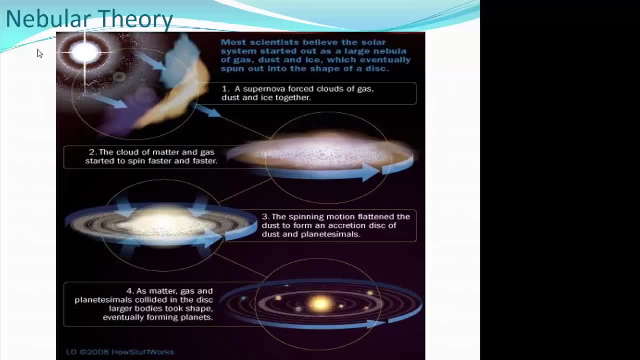 Meaning some long ago exploded star, maybe even gas and dust that came from the original big bang floating through the universe. And as that gas and dust began to clump together, The gravity that the mass of that dust and that dust created, That gravity of all that clumping together, began to force more mass and dust together. 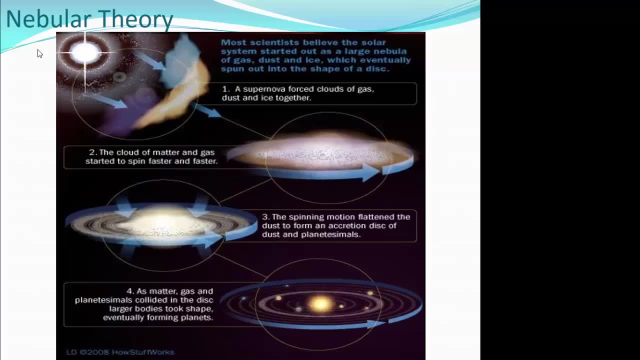 Until it clumped together into a cloud of matter and gas. that began to sort of spin around itself And the spinning motion flattened that cloud of dust and gas out And at the center, where most of the dust and gas was, The gravity got high enough to clump it together into a bigger and bigger object. 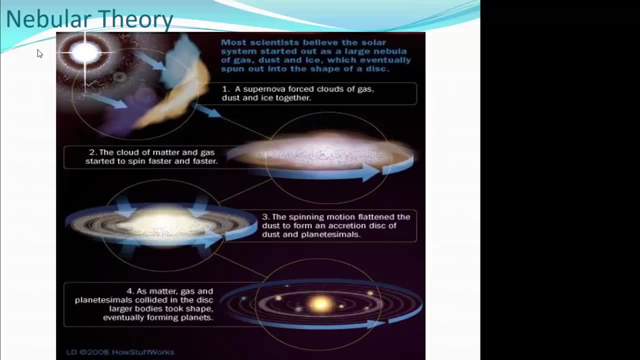 That eventually became the sun, And out on the edge of that disc The dust and gas clumped together to form the planets. So as the matter, gas and planetesimals collided in that disc, The larger bodies took shape And they eventually formed the planets. 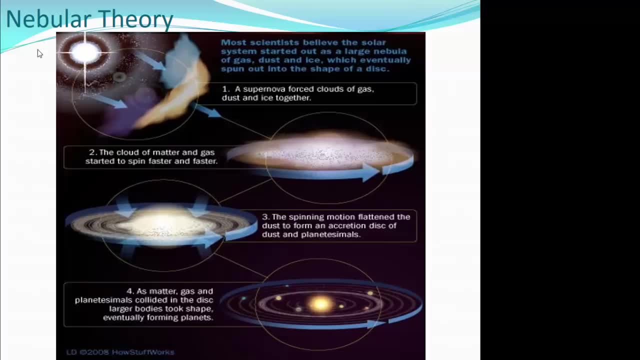 So what the solar nebula theory tells us Is that large clouds of gas and dust condensed into solar systems, And that process happened essentially at the same time When the sun got big enough and heavy enough That its mass was able to force the first hydrogen into helium. 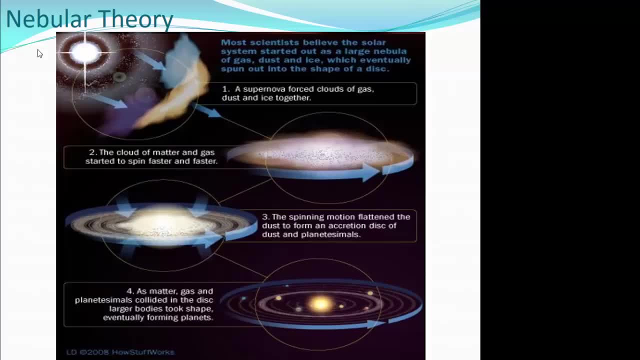 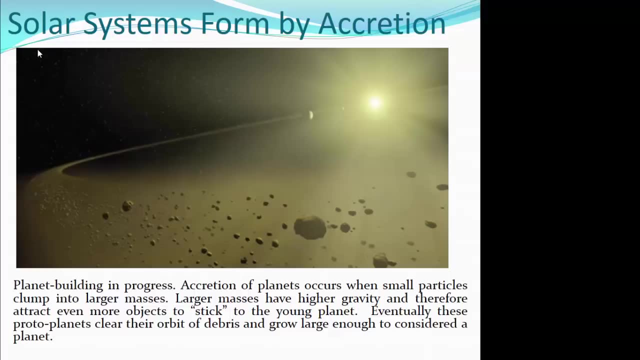 That is when the sun literally turned itself on And began to become the fusion engine that it is And began to radiate light and energy away from itself. At the same time, the planets were forming. The planet building process is a process of accretion. 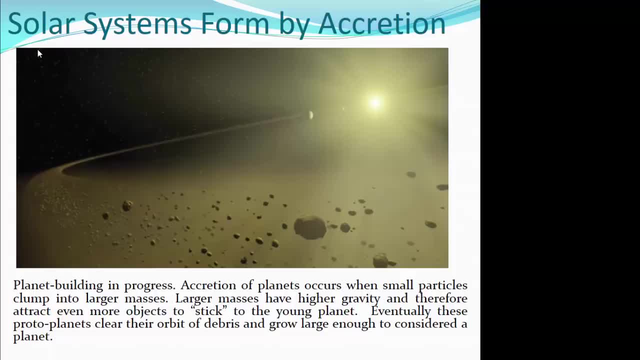 As the solar nebula begins to spin And the disc flattens out And the sun With its greater and greater mass Turns itself on and becomes a fusion engine. All that rocky debris, All that other gas and dust Is spinning around the solar system center. 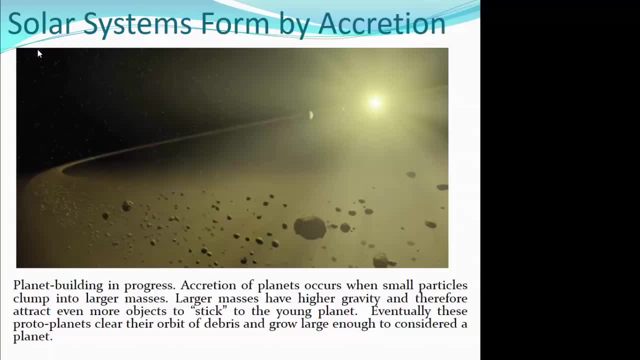 That very young sun In an orbit around the sun. Well, as those larger masses with greater gravity Begin to pull in smaller masses, They begin to attract Or actually stick or clump together And eventually larger and larger masses are formed In individual areas around the sun. 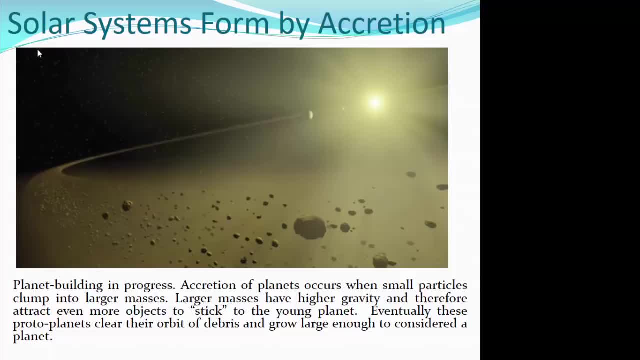 Individual orbits around the sun And as they grow larger and larger, They become known as protoplanets Or young planets Or sometimes even planetesimals. As those protoplanets grow larger and larger, Their gravity becomes larger and larger And they pull more of that dust and debris. 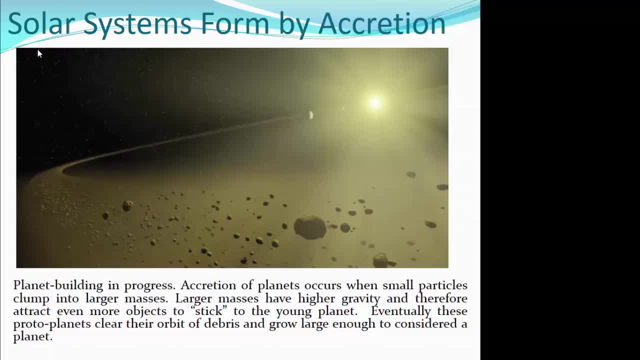 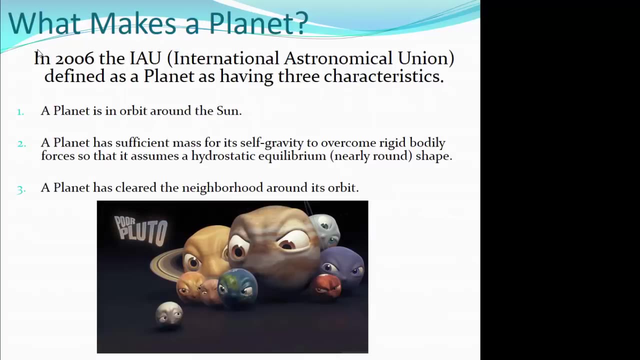 In their particular orbit And it all clumps together in a big one chunk. Eventually, That protoplanet will sweep its entire orbit Clear of all debris and gases And it will all be clumped together in one planet In 2006.. 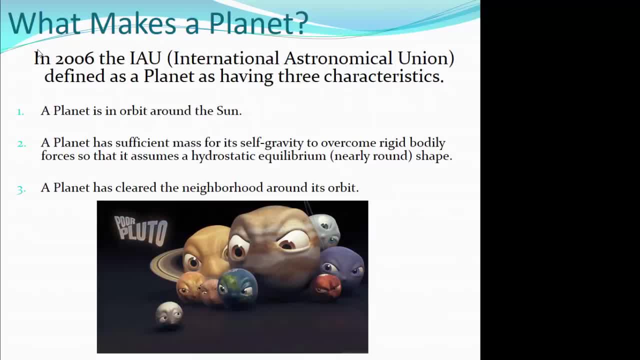 The IAU, The International Astronomical Union, Defined a planet As having three characteristics: A planet is in orbit around the sun. Okay, A planet has sufficient mass Meaning. it's big enough That its gravity is large enough That it will overcome rigid bodily forces. 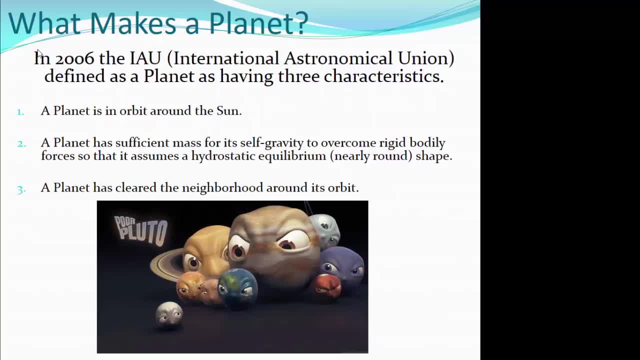 That means all those rocks and stones And huge chunks of asteroids That clump together in kind of an irregular shape. If the optic is big enough To become a planet, To be considered a planet, Then the gravity is high enough, Strong enough. 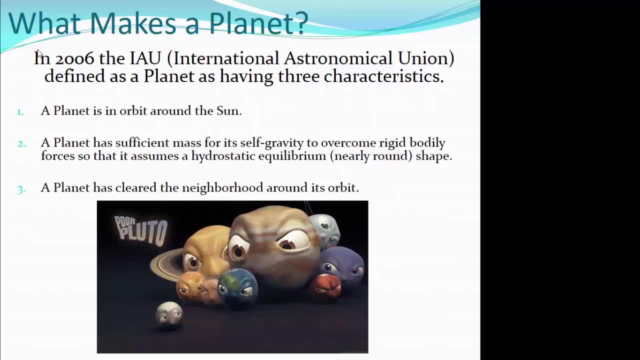 That it overcomes rigid bodily forces And assumes a hydrostatic equilibrium. Well, a sphere is the most stable shape known, And that's why eggs are close to being spheres. It's the most stable shape known. So Hydrostatic equilibrium Meaning pushing out. 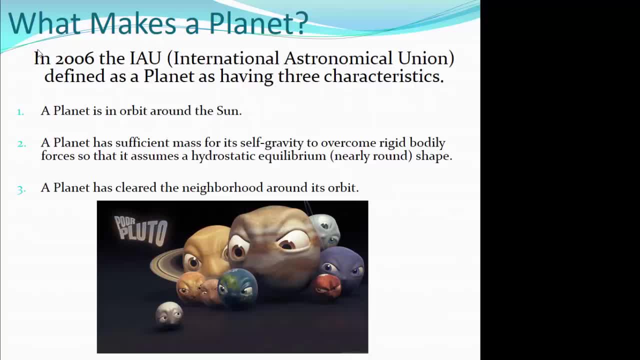 Is equal to the pulling in, And it assumes a round shape Or a globe shape. So a planet has to be big enough That its gravity, Its own gravity, Is forced into the shape of a globe. A planet also has to have cleared its neighborhood. 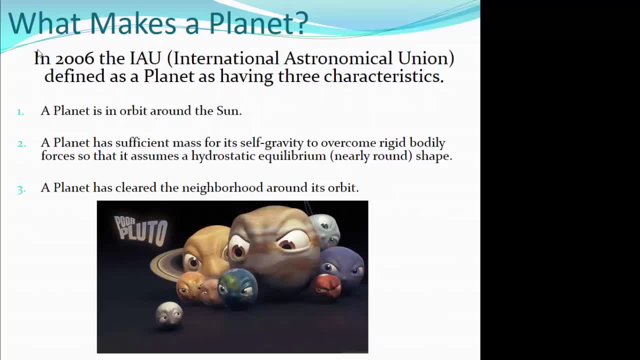 Around its orbit Of all other debris. So all of the planets That we think of Are planets, except for Pluto. What we see when we look at Pluto Is two things. One: Pluto isn't exactly In that flat disk. 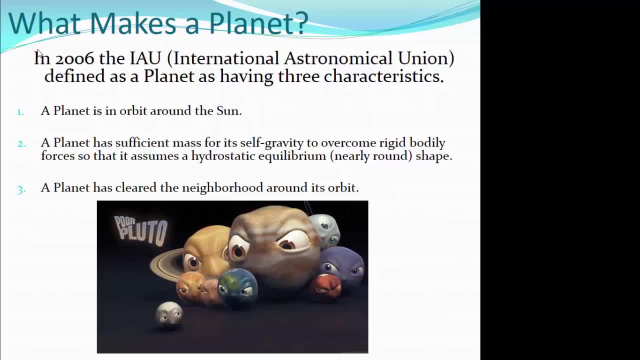 Its orbit is actually widely skewed From the rest of the planets And It's actually not large enough To have cleared its neighborhood Of debris. There are other large objects In and around Pluto. So, As of right now, Pluto. 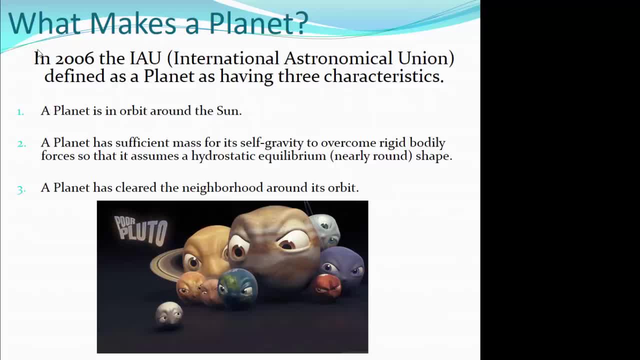 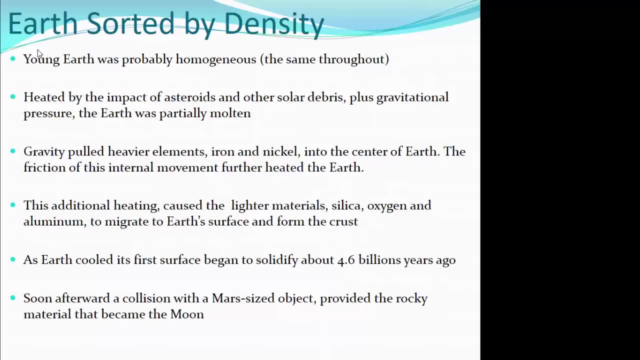 Is no longer considered A planet. So the young earth Has now developed Around that young sun And the first earth. The young earth Has developed Around that young sun And the first earth. The young earth Has developed. 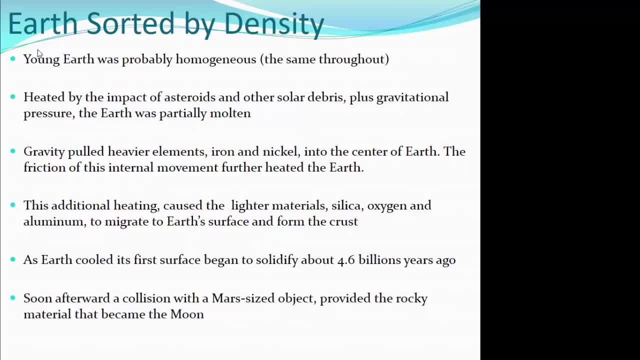 Around that young sun And the first earth. The young earth Has developed Around that bright earth From the past earth. The young earth Was probably homogeneous, Homo Meaning The same, And so it was the same Throughout. 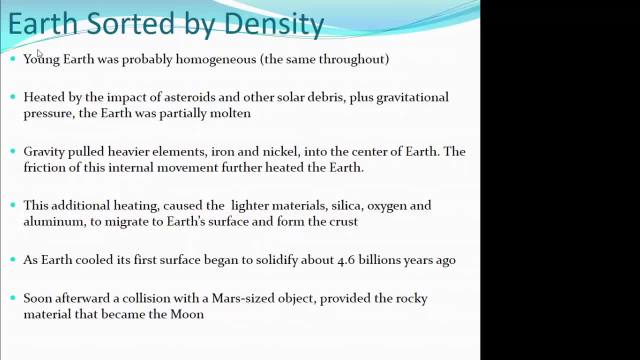 Homogeneous Meaning The same Throughout: A bunch of rocks, A bunch of elements, Some ice, Some water, But pretty much the same Throughout During the first Billion Or So years, Maybe Almost two, But 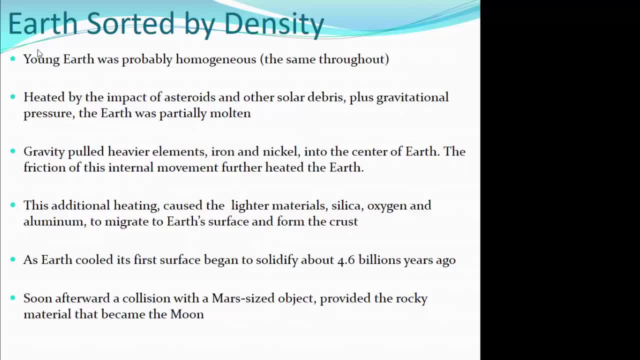 Billion Or So years, As with the debris in its orbit, but it was also colliding with other objects that were in the solar system. during this impact of asteroids and other solar debris, plus its own gravitational pressure as it became larger, the earth heated up and it became partially molten as it became. 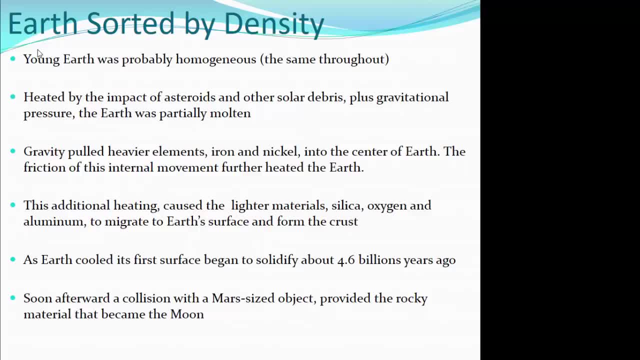 partially molten. gravity pulled heavier elements such as iron and nickel to the center of the earth. the friction of this internal movement, those elements rubbing together, literally further heated the earth. so this additional heating caused lighter materials, materials, silica, sand and oxygen- and aluminum. there's a lot of aluminum in our crust. all those lighter materials migrated. 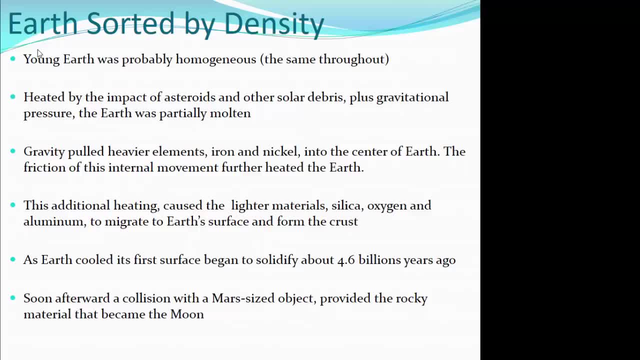 to the earth's surface and that's what formed the crust. so the crust was solid. the, the center, the mantle, was more plastic. actually, the mantle is more like soft candle wax and of course, we think that the- uh, the core, is partially liquid and partially solid and it's 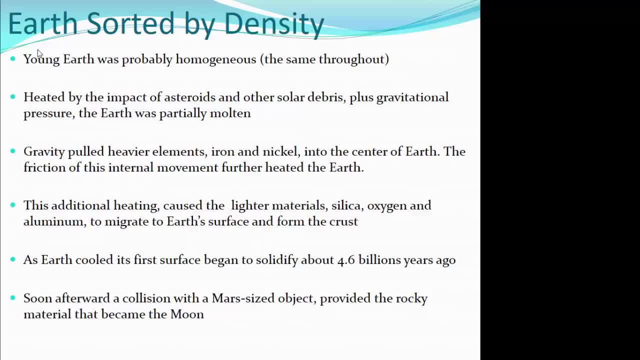 the solid spinning within the liquid that actually helps give us our magnetic field. nonetheless, the earth cooled and that first surface began to solidify about 4.6 billion years ago. how do we know that? well, we have fossil records. very few, but a few fossil records that date that far back. 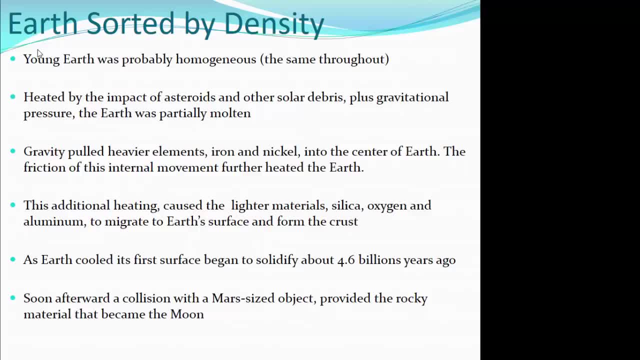 giving us indication that the earth is about 4.6 billion years old, soon after that first formation. theoretically it is now thought that a collision with a marsed side object smashed into the earth all the interior of the earth kind of blew out into space and all. 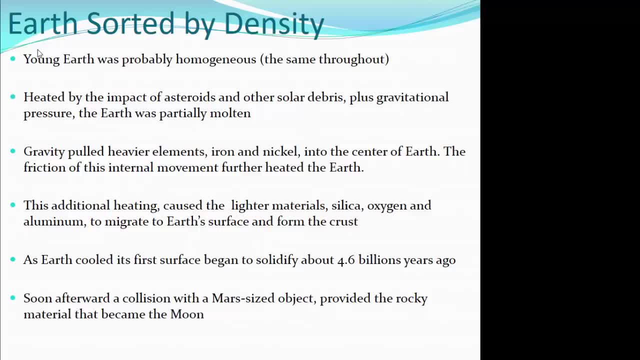 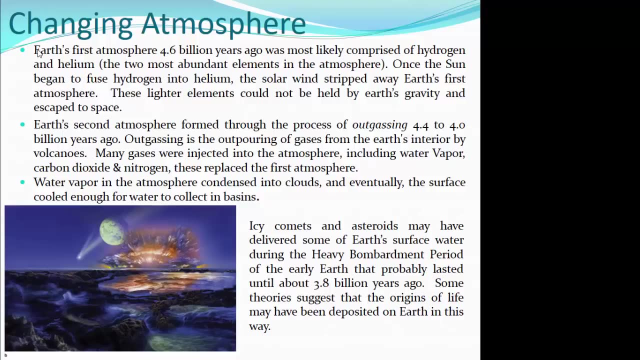 that rocky material that blew out into space from that collision with that mars size object became the material that clumped together and formed our moon. so the atmosphere, first atmosphere very likely was that hydrogen and helium that makes up most of the universe, but that's very, very light. 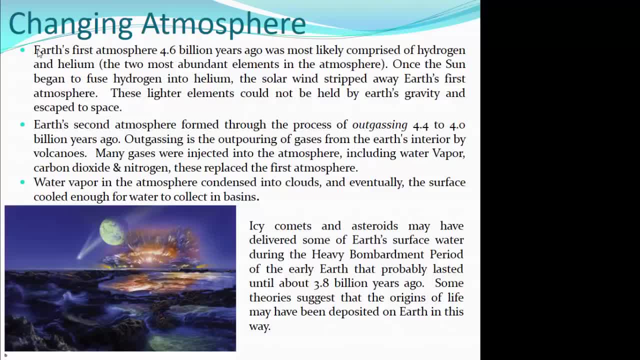 and the solar wind, meaning the radiation that came from the sun. as the sun began to burn, that solar wind very likely stripped that hydrogen and helium away from the earth's surface. so the first atmosphere about 4.6 billion years ago, very likely that hydrogen and that helium two. 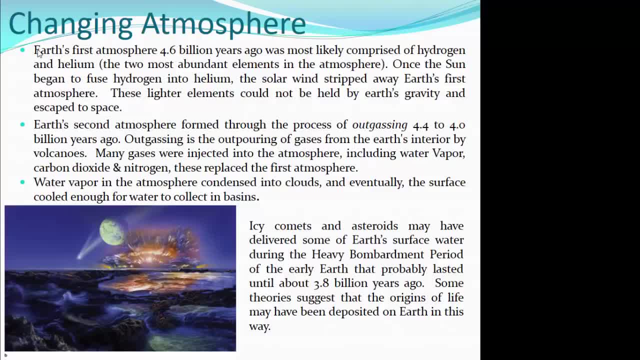 most abundant elements in the atmosphere. once the sand, the sun, began to fuse hydrogen and helium together, that radiation that moved out away from the sun is considered the solar wind and the lightness of those elements and that solar wind stripped that first atmosphere away. these lighter elements could not be held by earth's gravity. they escaped into space, the second atmosphere. 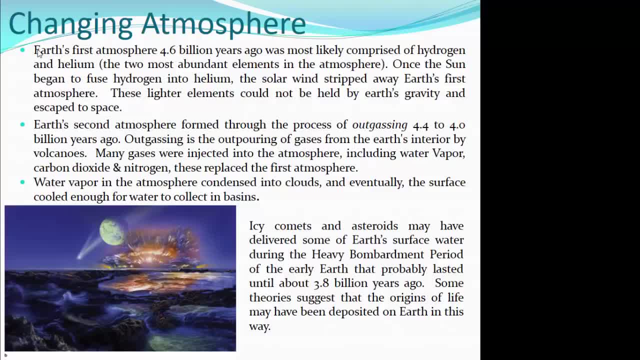 that's right. there's two and we're going to find out actually a third, the atmosphere we live in being the last. the earth's second atmosphere formed through a process of outgassing between about 4.4 and 4 billion years ago. outgassing is the outpouring of gas into the atmosphere, which is 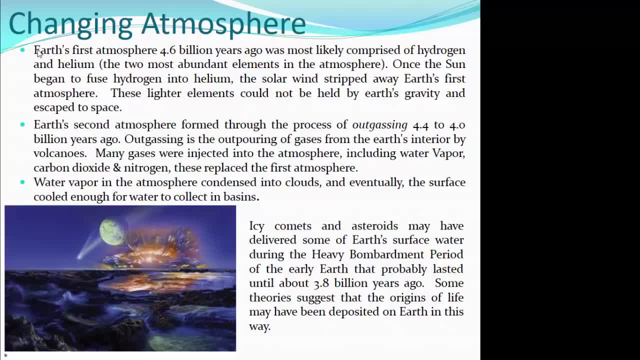 of gases from the earth's interior by volcanoes or volcanism. all of the movement of the earth, the earth's crust, the plates rubbing against each other, plates moving away, plates colliding, spaces opening up, and just volcanism in general. the volcanoes on the earth poured out gases. they 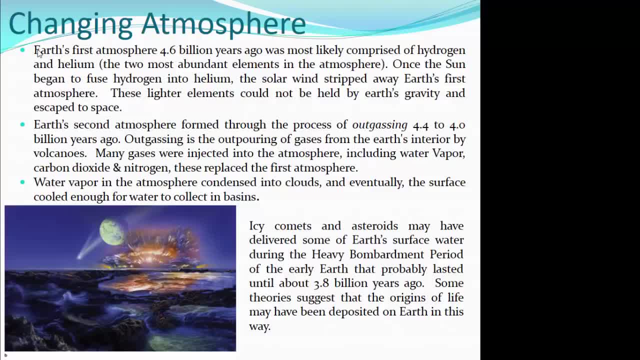 were injected into the atmosphere and they were water vapor and carbon dioxide and nitrogen. and those three vapors- vaporous water, carbon dioxide and nitrogen. they replaced the first atmosphere. notice: no oxygen there. the earth was far enough away from the sun that, unlike venus, water is able. 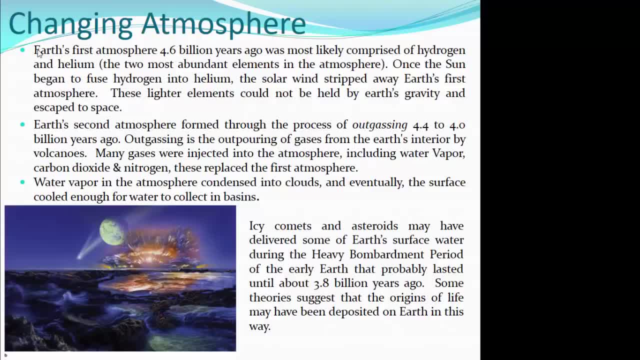 to condense into clouds and rain and eventually the surface cooled enough for water to collect in the basin. not the case at all with venus. venus is too close to the sun. it never cooled down. all that water vapor remained gaseous, and water vapor is an excellent greenhouse. 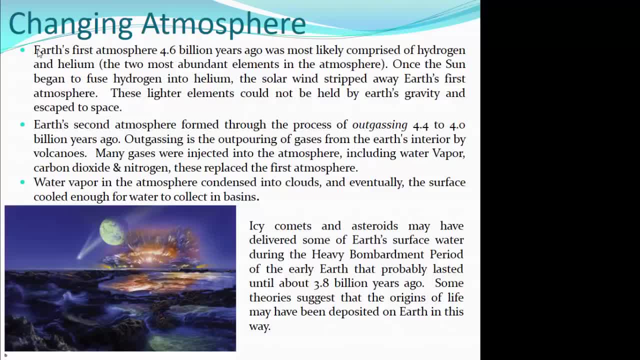 gas and one of the reasons why venus is so hot and caustic. it's also thought that icy comets and asteroids may have also delivered some of the earth's surface water during the heavy bombardment period of the early earth that probably lasted until about 3.8 billion years ago. some theories 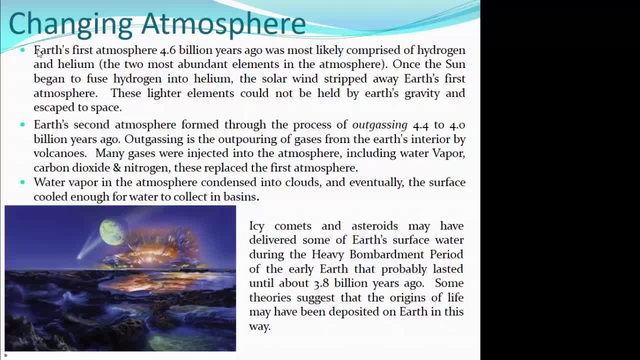 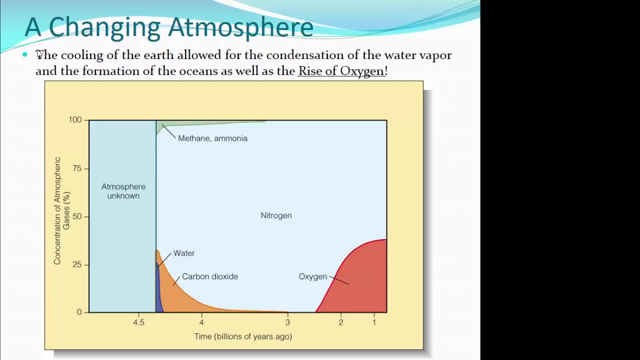 suggest that maybe even the origins of life on earth could have been deposited in this way, meaning single cell plants and animals may have been deposited on earth, and some of those icy chunks that hit the earth in that heavy bombardment period. the atmosphere of the earth, therefore, has been changing since the formation of the earth, the first. 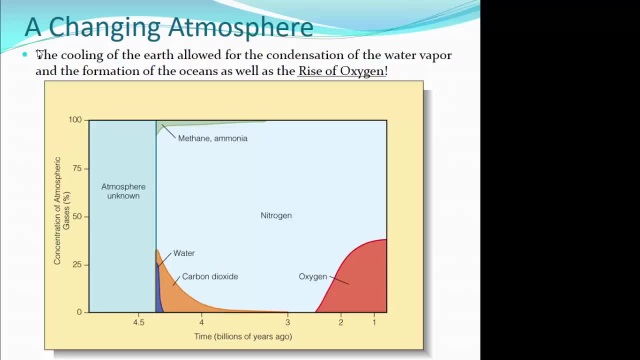 atmosphere- unknown but likely hydrogen and helium- then replaced through outgassing sometime 4.3 to 4.4 billion years ago. that's when the outgassing began. during that heavy bombardment period, lots of volcanoes, lots of tectonics, lots of explosions, lots of energy and water vapor. 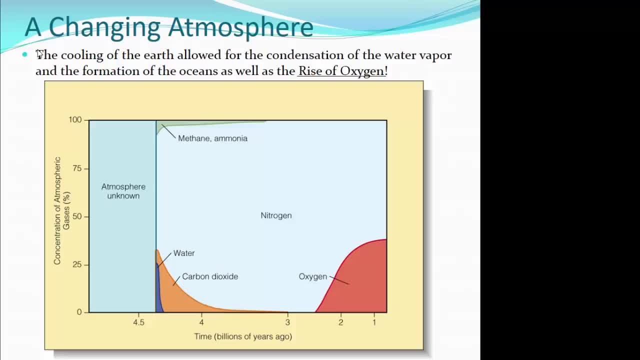 released into the atmosphere: carbon dioxide, ammonia and plenty of nitrogen. and then, at some point, around 4 billion years ago, maybe shortly before, the first blue green algae show up on the earth's surface, those are plants, and plants take in carbon dioxide and release oxygen. well, the carbon dioxide begins to be pulled down and oxygen 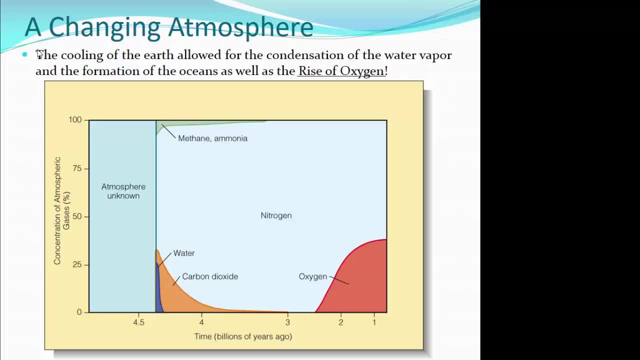 release. but you see, it doesn't get into the atmosphere as free oxygen until about 2.3 to 2.5 billion years ago. at first the oxygen is attacking other elements, so attacking iron in the form of carbon dioxide, rust, and that's when we see those red rocks. eventually there's enough oxygen that we saw the rise of oxygen from about 2.2 billion. 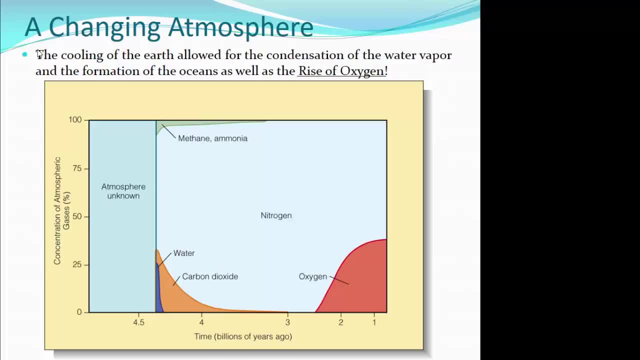 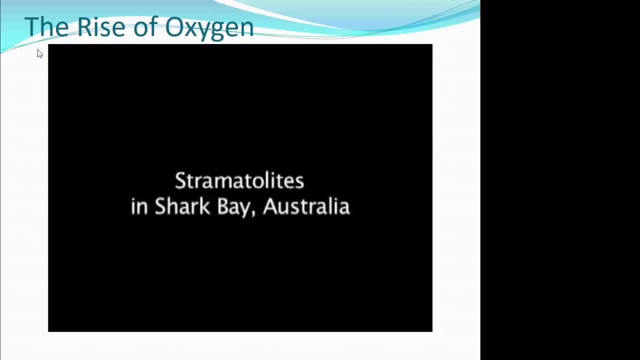 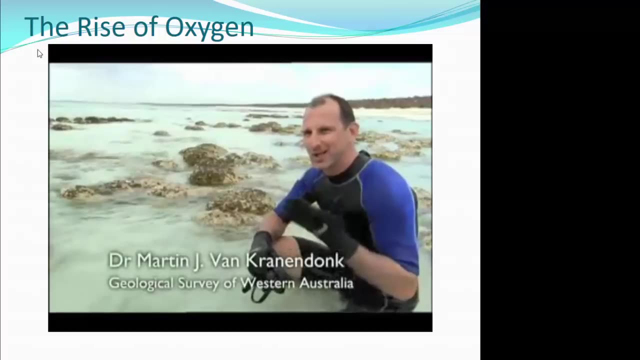 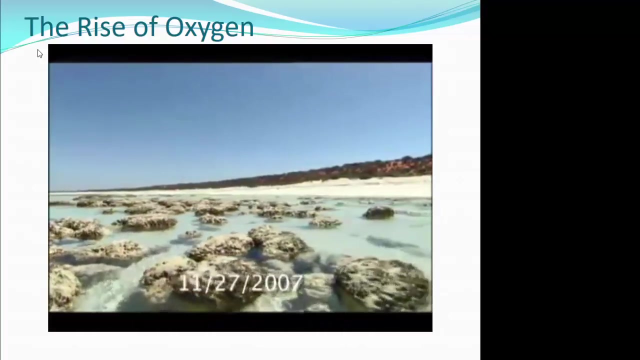 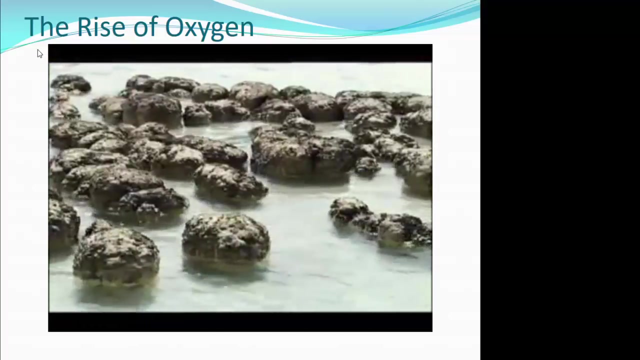 years ago up to its current level today. Cフ chief v T R e h n r. And they're found only in a few places in the world, and the best place on earth to see them is right here in Shark Bay. The top layer is actually made up of millions of microscopic organisms. 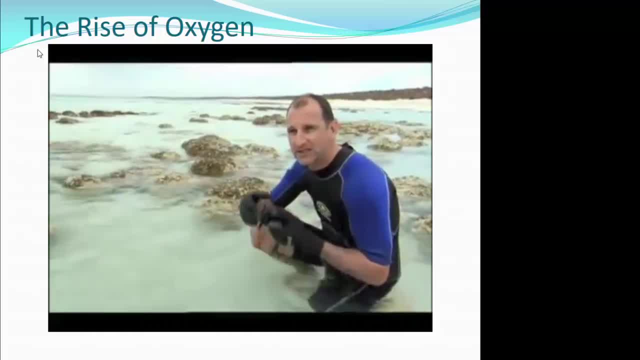 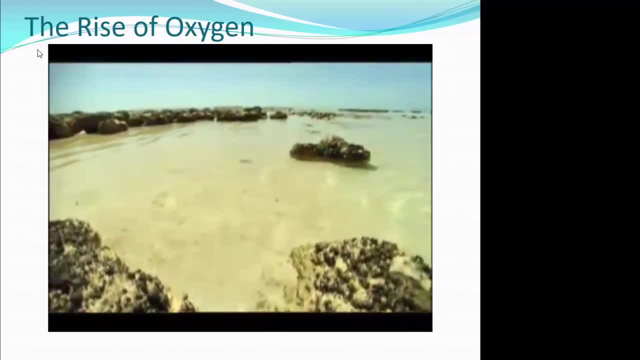 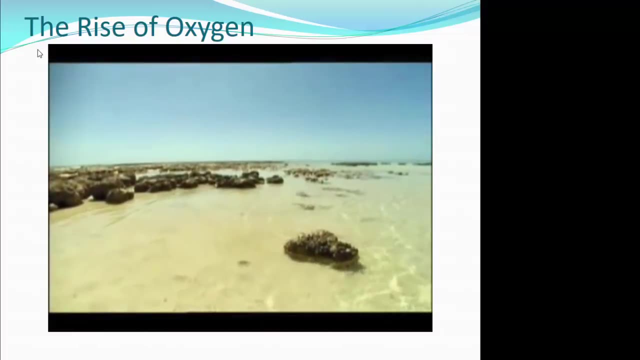 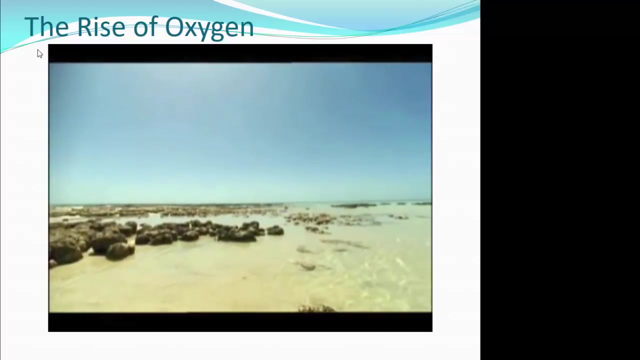 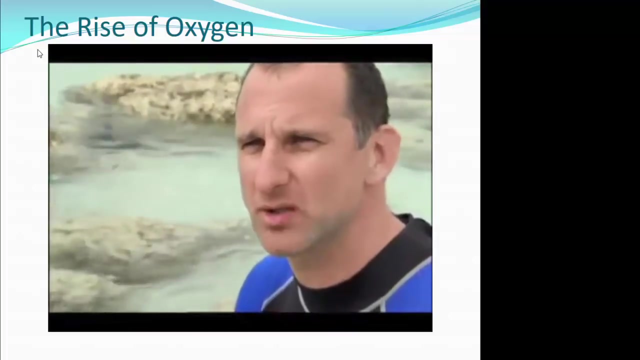 Mostly a type of bacteria called cyanobacteria that gets its energy from sunlight. these bacteria did something extraordinary As they took in sunlight and photosynthesized. They broke the chemical bonds in water, Releasing something that would completely change the planet: They released oxygen. Stromatolites are really special because they were some of the first organisms to produce oxygen, and not just in a small amount. 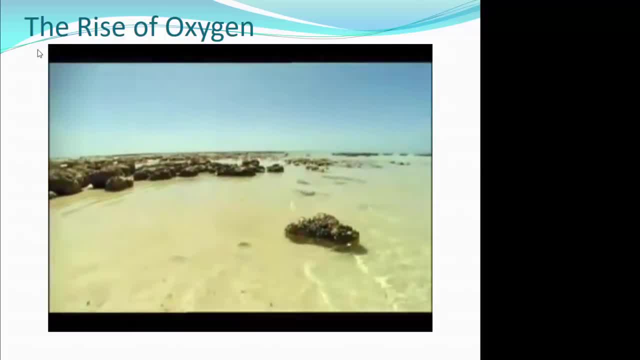 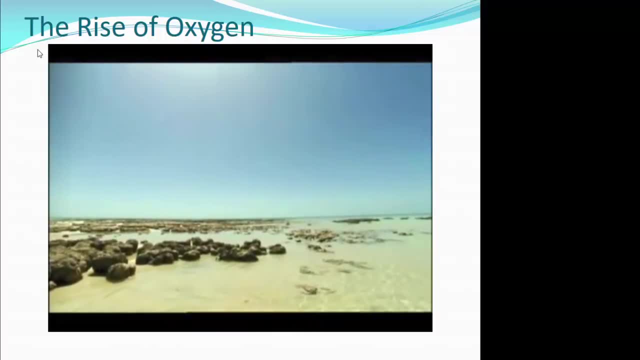 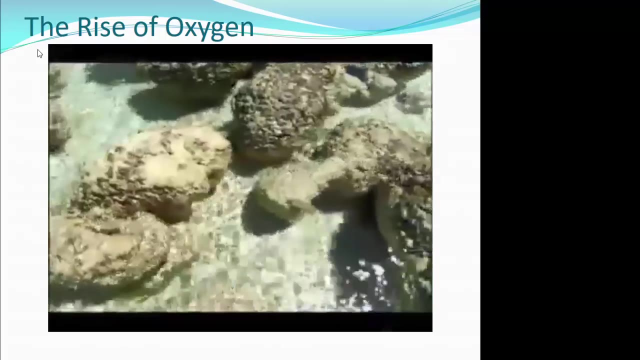 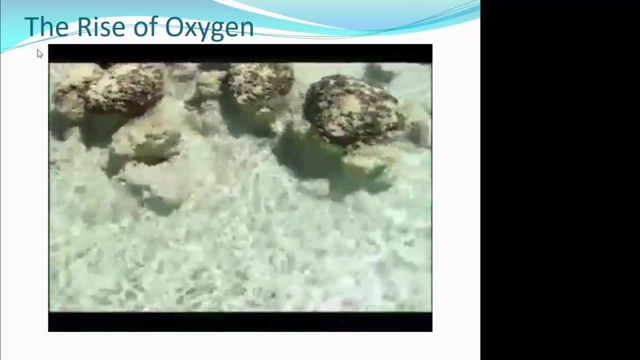 By around two and a half billion years ago. Stromatolites covered all the ocean shallows worldwide, and all of them were pumping out oxygen. This was to lead to some of the most profound changes in the history of the earth. Ultimately, the planet would have an atmosphere rich in oxygen. 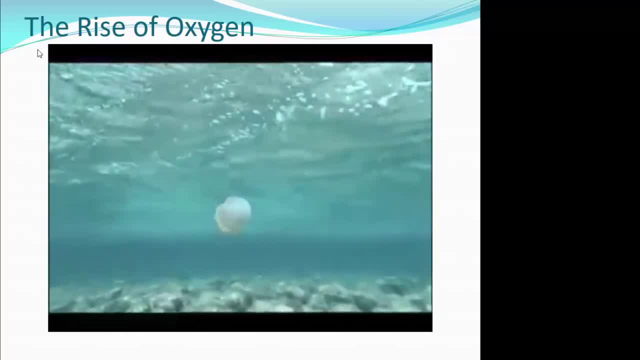 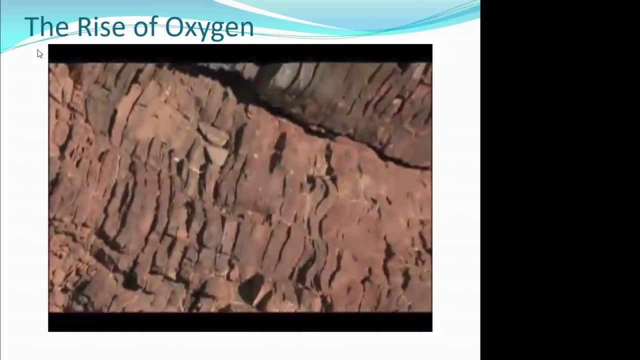 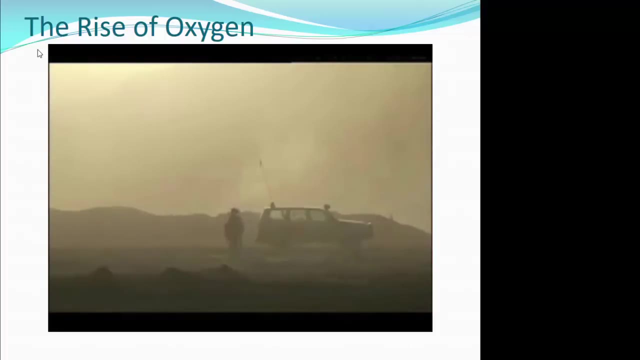 But before that could happen, something got in the way. Two and a half billion years ago, these rocks were formed deep beneath the sea And they hold the key to what happened to the oxygen bubbling out from the stromatolites. Back then, the seas were rich in iron that was dissolved in the water. 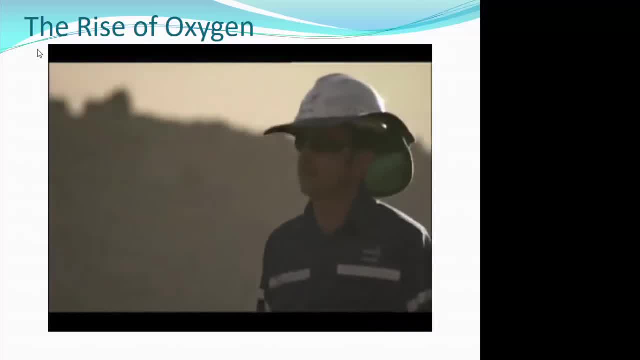 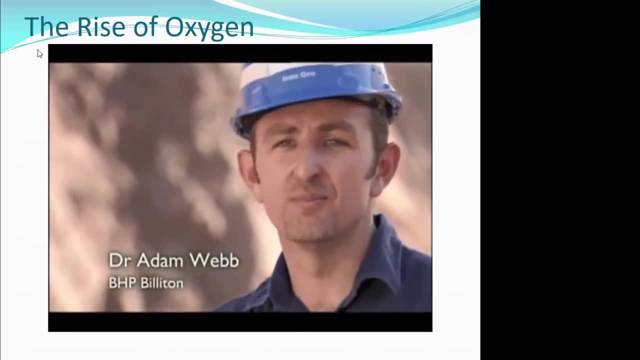 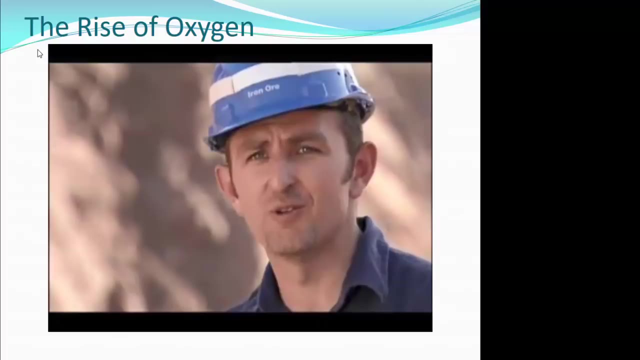 Adam Webb is a geologist who has Studied this ancient period in Earth's history. It says those oxygen levels started to rise in the ocean from the stromatolites. It mixed with and reacted with the iron and basically rusted, and it's this rust that settled on the ocean floor. 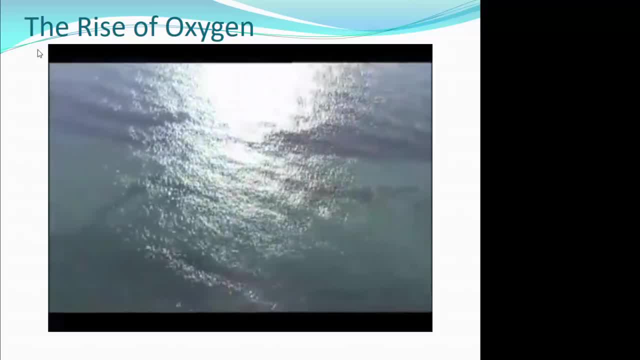 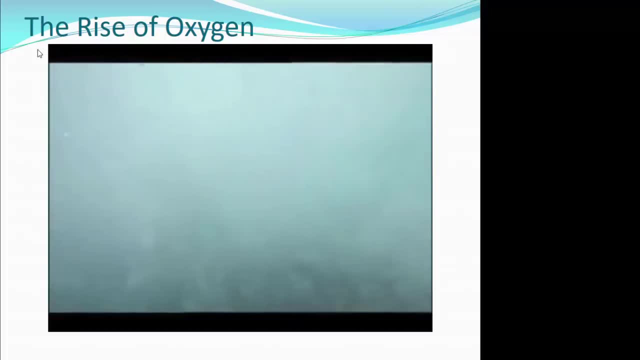 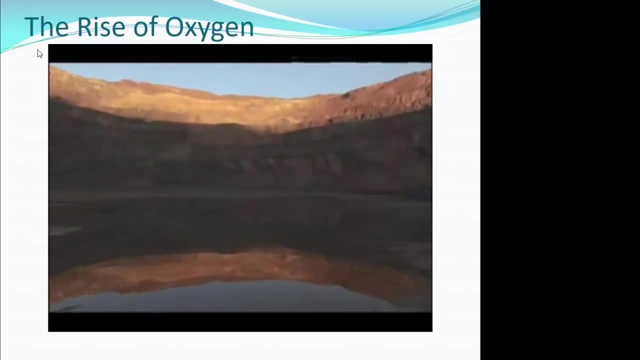 It was this reaction that stopped the oxygen from leaving the ocean. The layers of rust were laid down all across the world, eventually turning into seams of iron and then into ore. Huge quantities of it can be seen in thick layers all around this mine As the iron rusted and this material settled on the ocean floor. 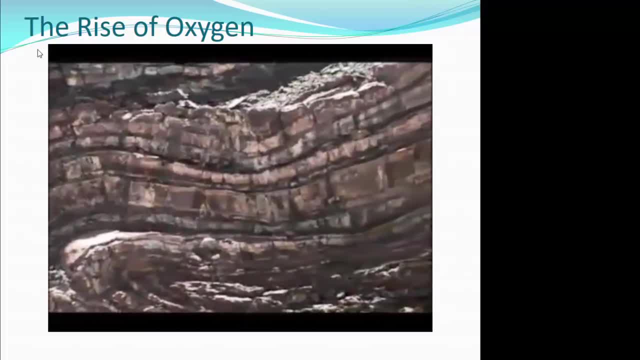 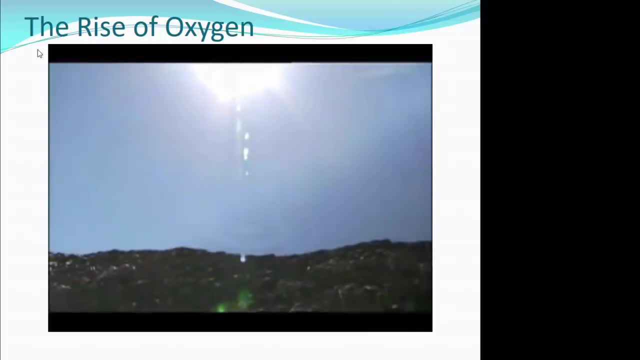 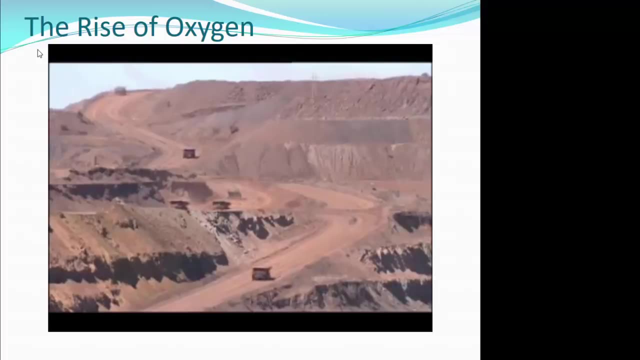 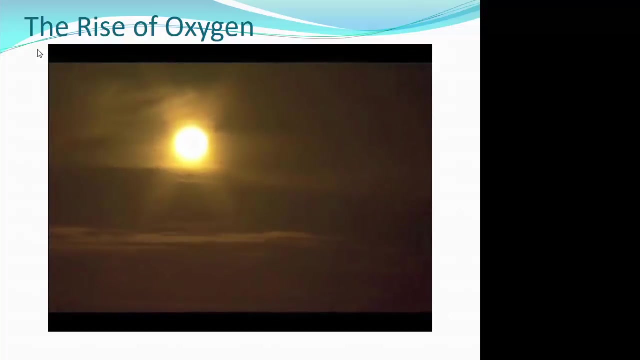 Layer after layer started to rise up and you ended up with huge, great big thicknesses of rock- exactly what we're seeing now today. The iron in the oceans had all rusted. there was none left for the oxygen to react with, So now there was only one place for the oxygen to go. It left the oceans and filled the atmosphere. 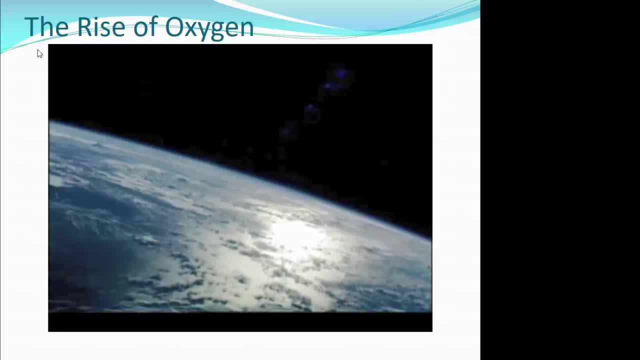 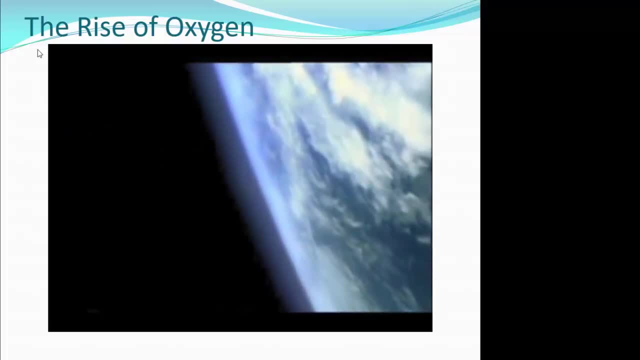 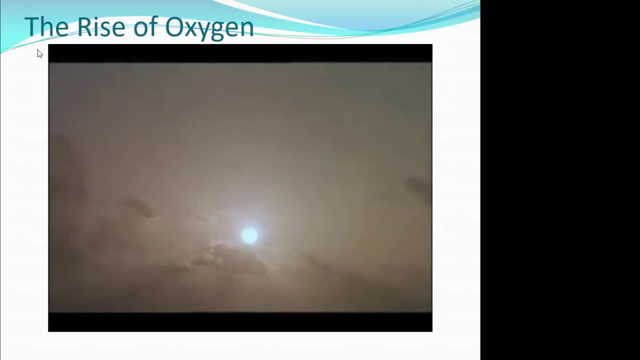 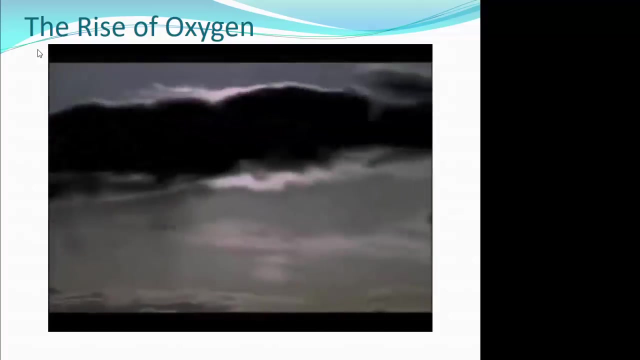 No event has been more important to the story of life on the planet. The first thing oxygen did was give the planet a vital protective shield. As oxygen rose through the atmosphere into the stratosphere, it formed a layer, The ozone layer. It shielded the planet from lethal ultraviolet radiation coming from the Sun. 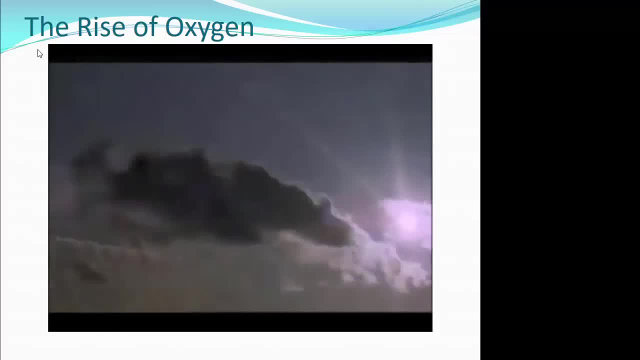 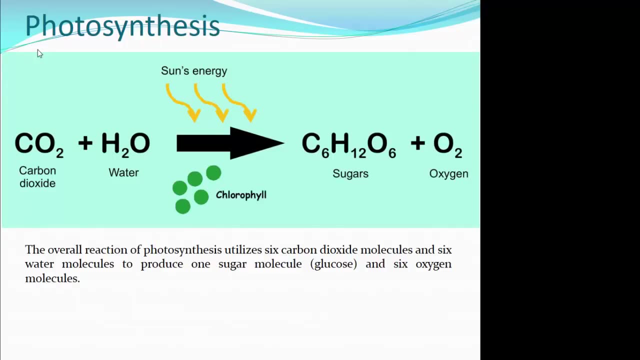 Allowing complex life to flourish on the surface of our planet. So photosynthesis. now I got these first blue-green algae. They have chlorophyll in them, They take the sun's energy, They take that carbon dioxide, They take that water and they will, and they create sugars or carbohydrates that they use to. 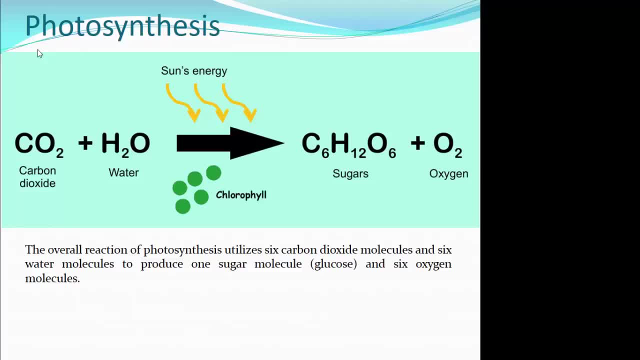 Grow and they release oxygen. the overall reaction of photosynthesis Utilizes six carbon dioxide molecules and six water molecules, produce one sugar molecule and six oxygen molecules. So where do we get the first oxygen photosynthesis? very likely Taking down the carbon and releasing the oxygen. Other ways that we got. 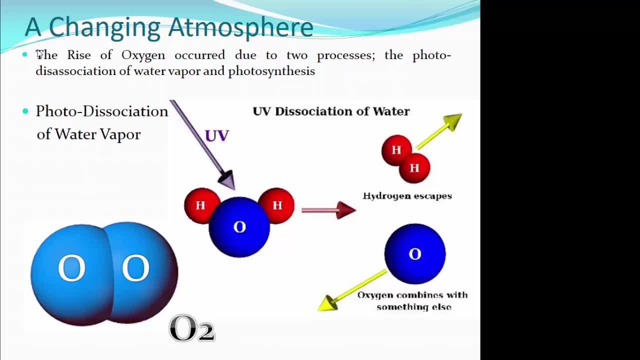 Oxygen in the atmosphere. Well, we had h2o, we had water vapor, We had h2o- that molecule in the middle, the one that looks like Mickey Mouse, That's your h2o. So what happened? the rise of oxygen occurred to two, due to two processes. 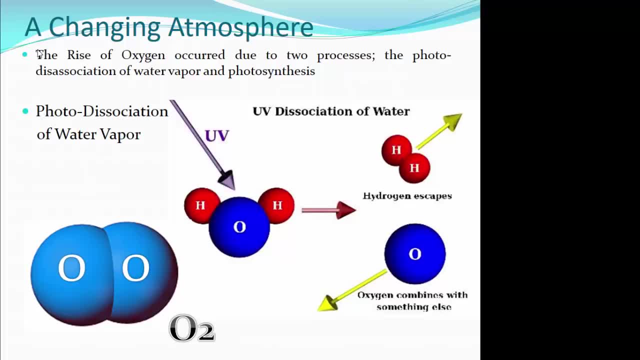 Photosynthesis, which we just looked at, and this other one, the photo disassociation of water vapor. Well, an association is a gathering things, so a gathering of things. So association of water vapor is the association of hydrogen and oxygen, h2o. Disassociation is the breaking that up. photo refers to light, So look at that purple arrow. 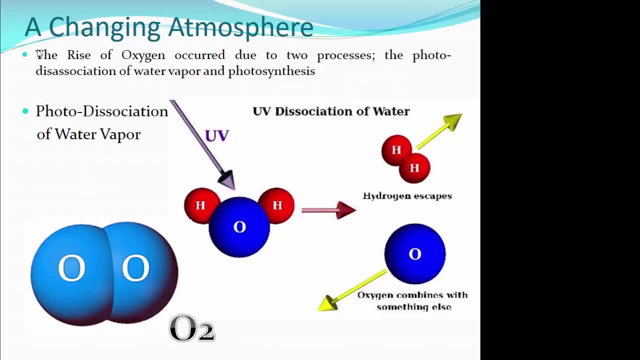 That is the UV light of the Sun coming in And banging into that water vapor molecule in the atmosphere. It's floating around, Mickey Mouse, all happy. UV ultraviolet rays which, as we know, burning rays, they're dangerous. They bang into that molecule, They split it apart. 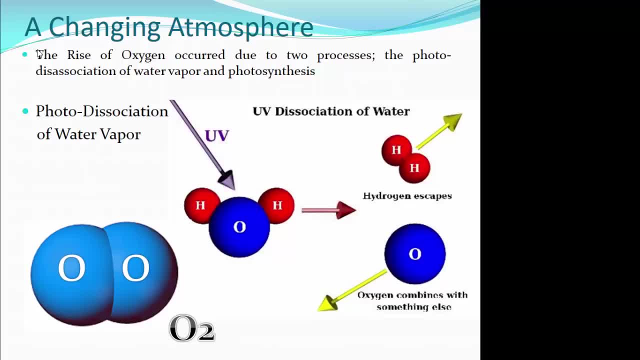 The hydrogen escapes into the atmosphere. but oxygen wants to combine with something else. It always combines with something else. oxygen is never by itself in the atmosphere, So it combines with another oxygen molecule, giving us o2. When you see oxygen tanks, they never say oh on them, they say o2, that's. 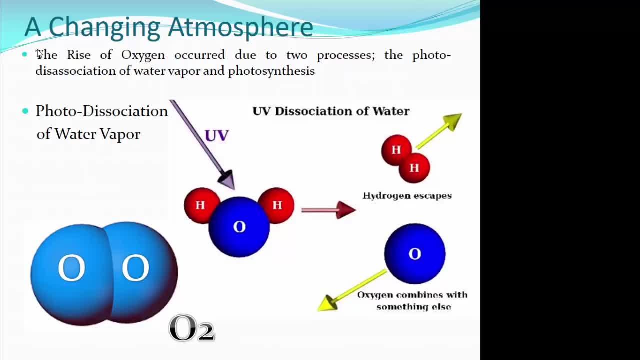 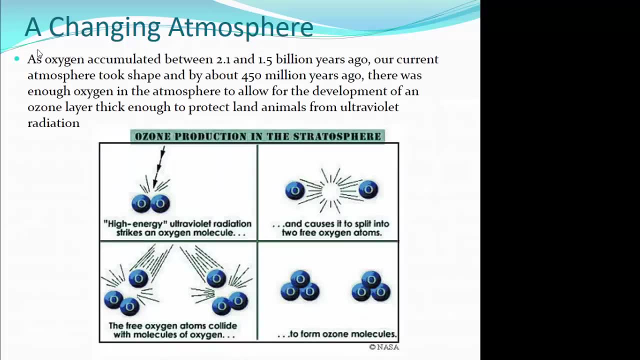 That we can breathe. so photosynthesis and the photo Disassociation of water vapor is what allowed for the rise of oxygen. from Now we also got ozone in the same way, where oxygen in the atmosphere was struck by ultraviolet radiation And that caused two free oxygen atoms to split, maybe joining with another oxygen. 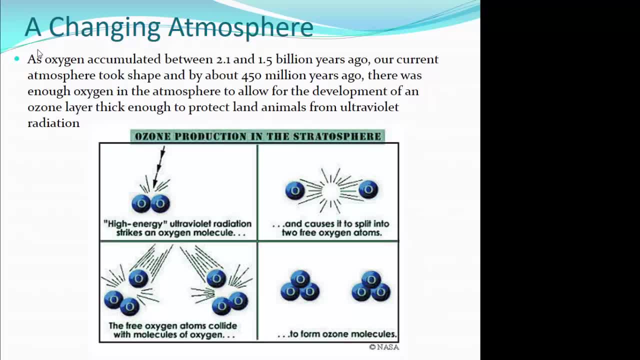 molecule to create O2, but possibly Joining with o2 to create o3 and o3. Well, o3 is ozone, so as oxygen accumulated between 2.1 and 1.5 billion years ago. Our current atmosphere took shape by about 450 million years ago. 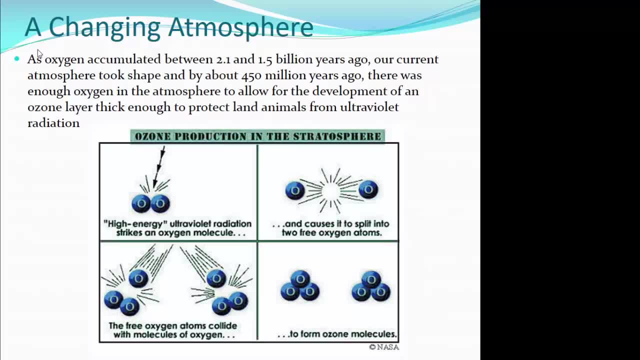 There was enough oxygen in the atmosphere to allow for the development of ozone O3 and a thick enough Ozone layer was enough ozone to protect the earth from UV rays to allow for the development of land, Plants and animals. prior to that, the UV is too bright, too strong. 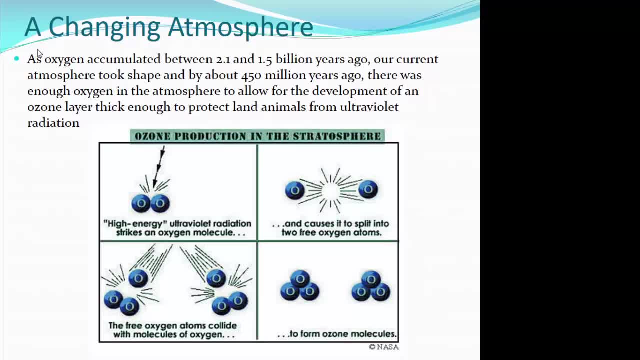 For land plant animals, so at about 450 million years ago. That is when we saw the development of land animals because UV radiation was being protected by the ozone layer. The composition of the atmosphere on the left of the permanent gases, the gases that are virtually in the same- 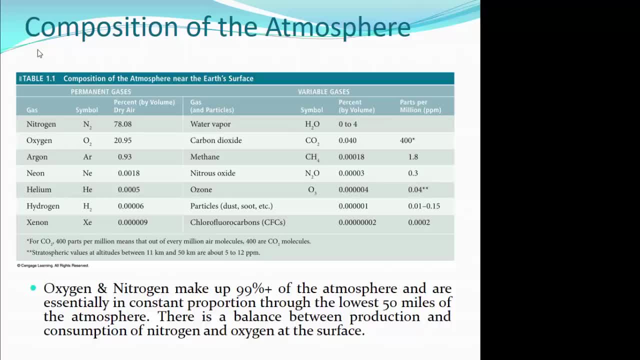 Proportion throughout the first 50 miles of the atmosphere. your your constant permanent gases: nitrogen, oxygen, argon-neon, helium-3 hydrogen and xenon. nitrogen at about 78% and oxygen At about 21%. when asked about the composition of the atmosphere, you need to know. 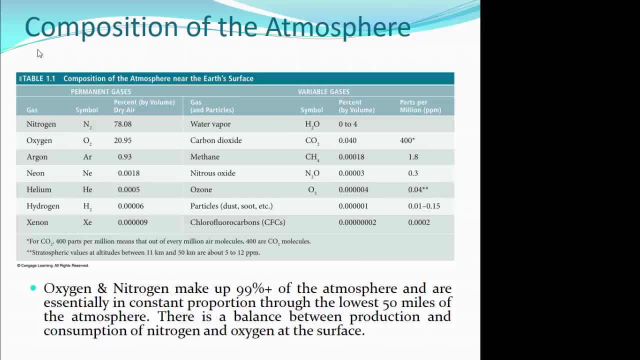 Nitrogen makes up about 78% and oxygen makes up about 21%. these other gases on the right- water vapor, co2, Methane, nitrous, nitrous oxide in o3. They're all in variable concentrations But very, very small. look how little o3. there is ozone, look how little nitrous and methane, and even co2- co2 now. 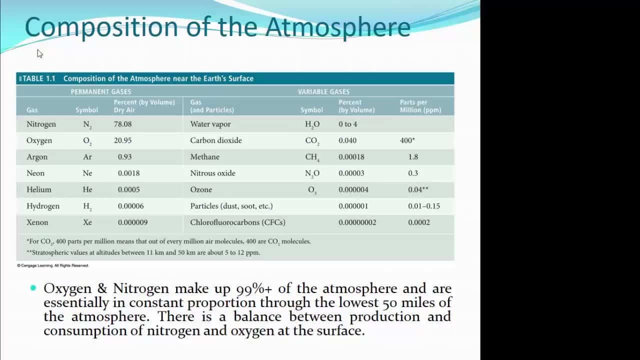 may be representing closer to 39, maybe even 4.04 parts per million. that amount of co2, as we all know, is increasing. and then water vapor. water vapor can vary between none and 4%. so this water vapor is highly Variable. and all those gases on the right, the variable gases, 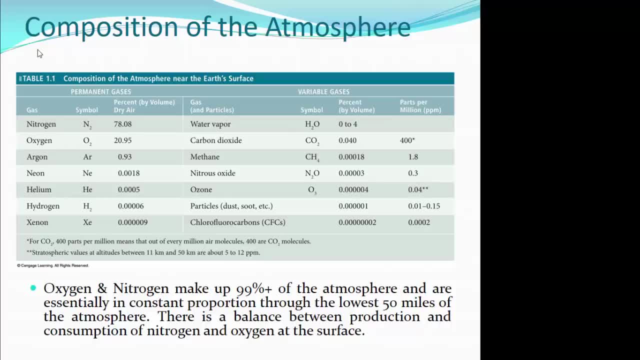 Those are all your, your greenhouse gases that would help us keep the earth warm, and there's way more water vapor than carbon dioxide. There's way more carbon dioxide than methane, and and that's on the rise because of farming, and nitrous is also on the rise as well. 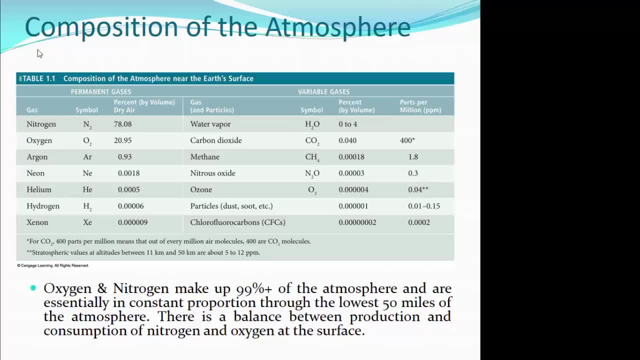 composition of the atmosphere. Oxygen and nitrogen make up 99 plus percent of the atmosphere and essentially in constant proportion, the lowest 50 miles of the atmosphere. There's a balance between the production of, and consumption of, nitrogen and oxygen at the atmosphere. Some it's created, some is destroyed, some goes into the ocean, some comes out of the ocean, some plants. 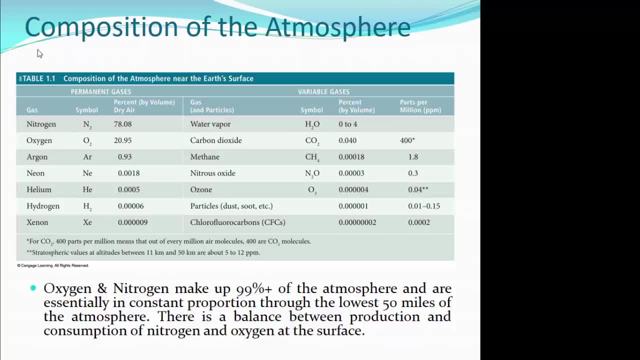 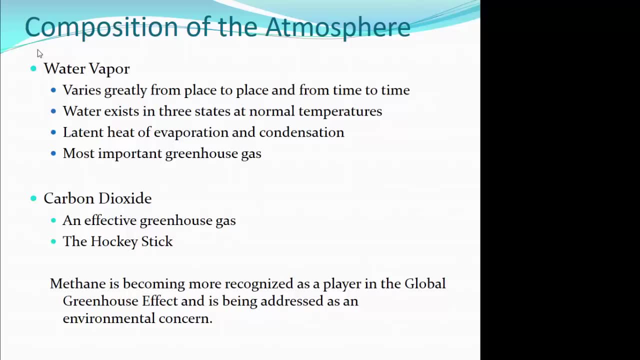 Release oxygen, they take in carbon dioxide. So there's this balance that is struck. Water vapor greatly varies from place to place and from time to time. It exists in all three states, as you know: liquid water and in gas. Water vapor releases and retains latent heat when evaporation and condensation occurs. 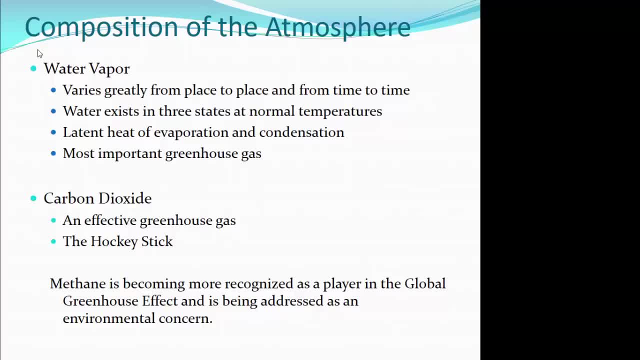 that's been very, very important to us. this concept of the latent heat of vaporization and the latent heat of Condensation- and, of course, water vapor, is the most important because of its abundance. greenhouse gas, carbon dioxide, is also an effective greenhouse gas, and the rise of carbon dioxide since the 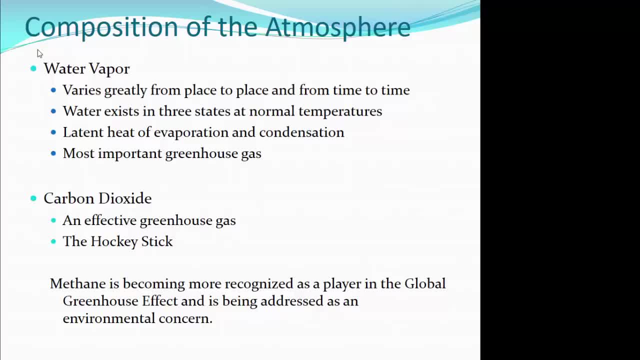 industrial revolution Is seen on the hockey stick Graph, which I'll show you in a moment. methane is also becoming more recognized as the player and the global greenhouse effect. It's being addressed as an environmental concern as well, But the biggest environmental concern we hear about, of course, is carbon dioxide. 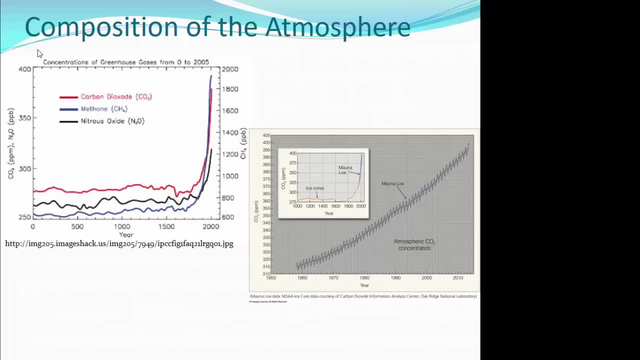 Here is the hockey stick graph, a graph of carbon dioxide, methane and nitrous oxide. now, These are three very important greenhouse gases, Not including water vapor. remember water vapor varies Constantly from place to place and from time to time, from between 0% to 4%. 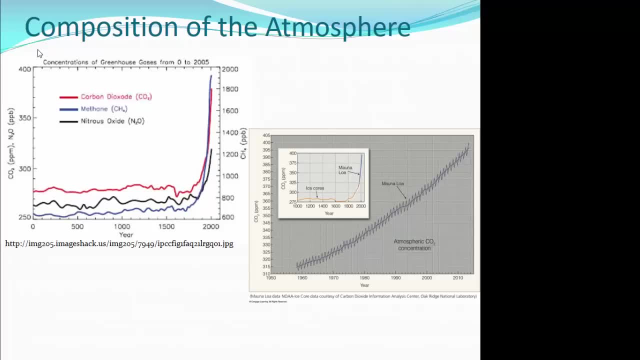 So these are just these, these gases that are less variable, There's less concentration in the atmosphere, But we see with the hockey stick graph this tremendous increase in the latter part way out on the x-axis. So going back 2,000 years, pretty constant proportions of those three gases through about the 1500s, in the 1600s. 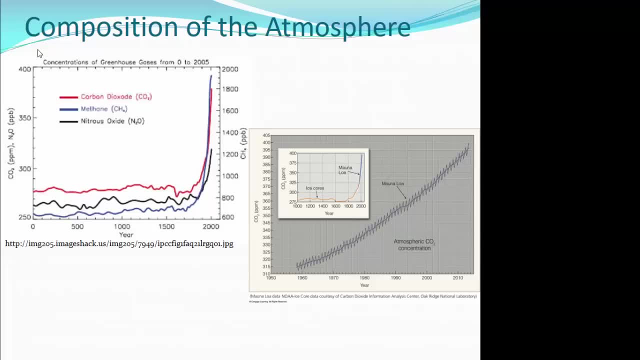 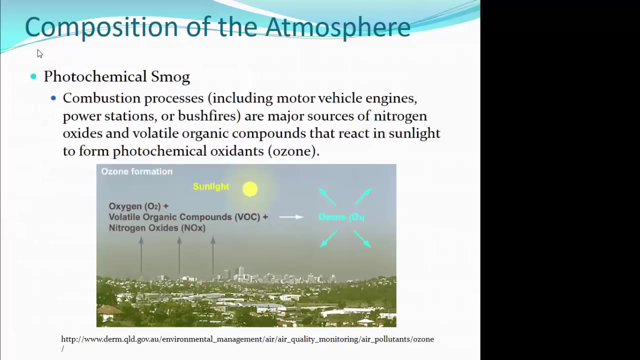 massive planting of trees in North America actually pulled down a Lot of the carbon dioxide, and then, during the Industrial Revolution, We see this tremendous increase after the 1860s of all three of these greenhouse gases and largely due to the burning of fossil fuels. Want to mention that photochemical smog. smog that we hear about is mainly ozone. ozone. 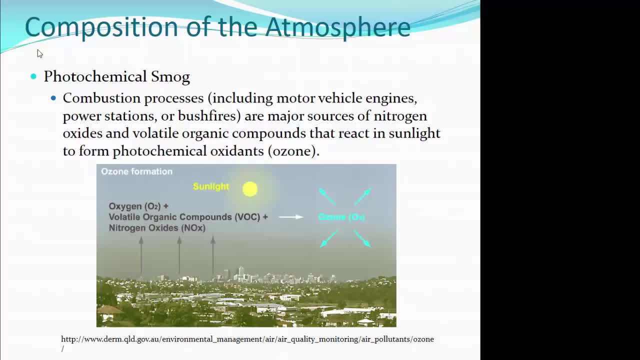 Combined with volatile organic compounds and nitrous oxides to create smog. So ozone at the surface is actually dangerous for us. us Ozone that protects us is up in the stratosphere, way up in the atmosphere. So ozone has kind of got two roles. 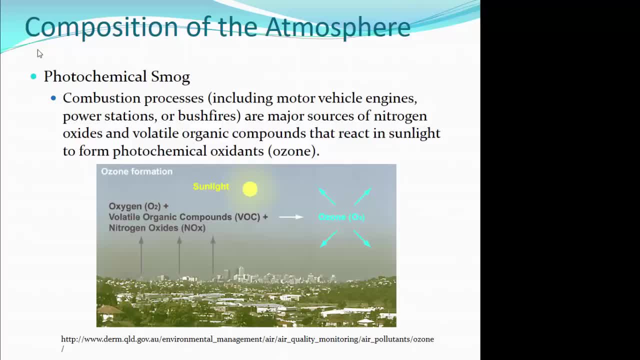 It's bad at the surface but very, very good in the upper levels of the atmosphere. Photochemical smog, combustion processes including motor vehicles, power stations and fires- all major sources of nitrogen oxides and volatile organic compounds. They all react in sunlight to form photochemical oxidants or ozone. 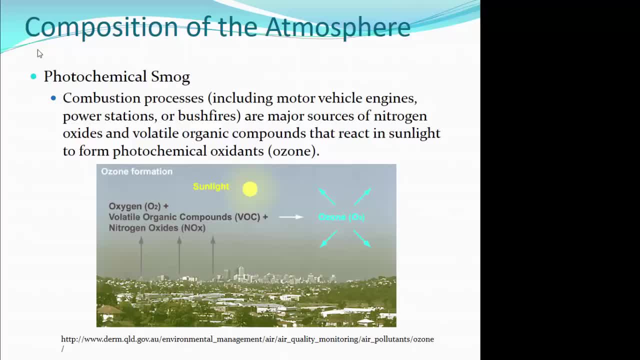 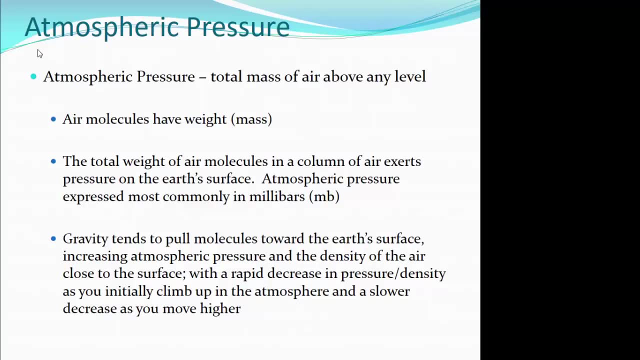 So ozone is good when it's way up there, but bad when it's down at the surface. So let's talk a little bit about what the atmosphere does. The atmosphere presses down on us. That's atmospheric pressure. You don't feel it. 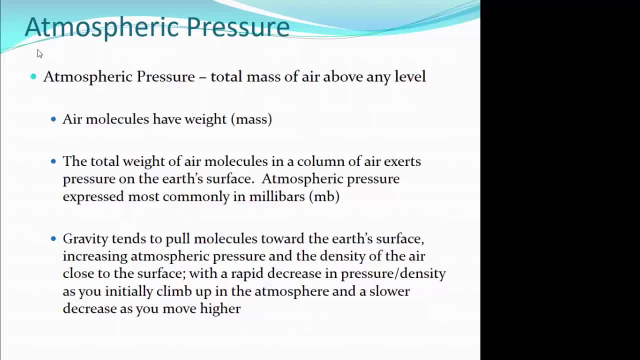 You're accustomed to it. But all those molecules, whether it's nitrogen, 78% oxygen, 21% carbon dioxide, water vapor, all those molecules, they have weight And all of that mass. of course, weight is a function of mass and gravity. 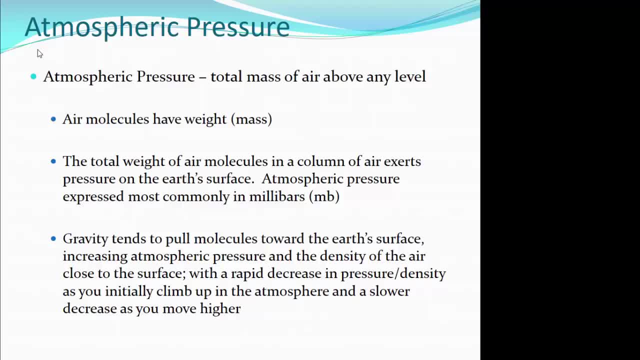 You know, you weigh less on the moon, right? Your mass is the same, but the gravity is lower. So mass and weight are not the same things, because weight is a function of gravity, The mass above any level. if I'm standing at the surface, there is a mass of molecules. 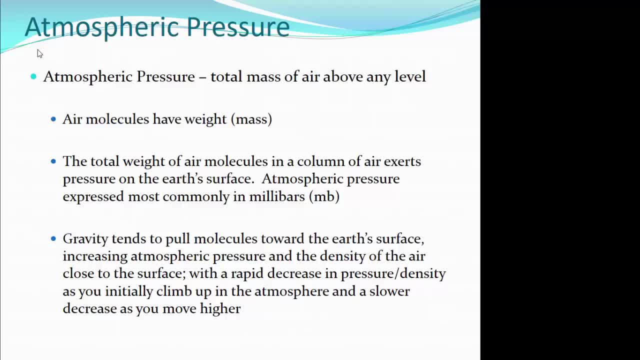 vaporous molecules above me, and the total weight of that mass equals the atmospheric pressure. Atmospheric pressure, all air molecules, whether they're nitrogen oxygen, carbon dioxide, water vapor, nitrous oxide, They all have mass Right. The total weight of the molecules in a column of air exerts pressure on the Earth's surface. 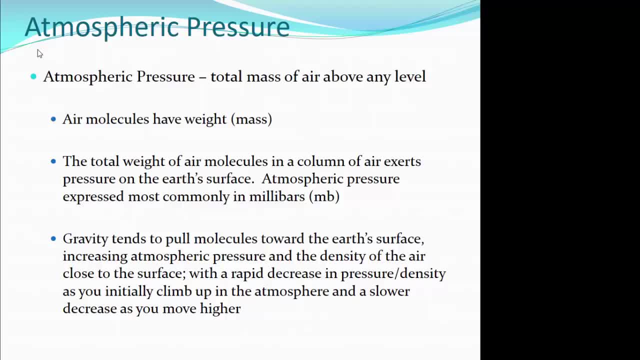 That atmospheric pressure is most commonly expressed in millibars. When looking at surface weather maps, atmospheric pressure is most commonly expressed in millibars. Millibars is just another way of saying pounds or liters. It's just a measurement of weight. 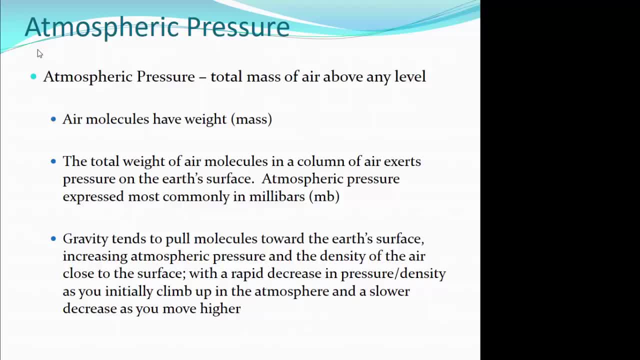 So all the mass above a certain level on the planet, that weight, because of gravity, puts pressure on the ground and that's atmospheric pressure. Now, gravity tends to pull the molecules towards the Earth's surface. That makes sense, right? The gravity is going to pull the molecules towards the Earth's surface. 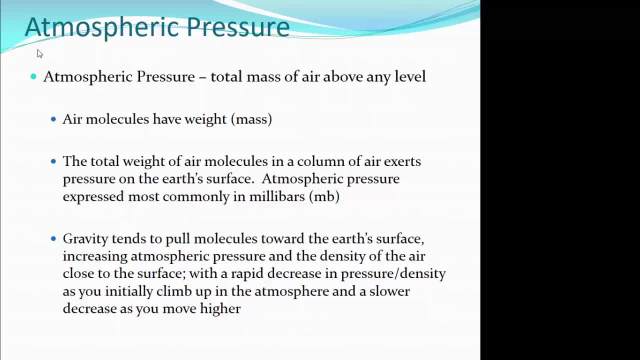 So there is increasing atmospheric pressure and the density of the air close to the surface, with a rapid decrease in pressure and density as you climb up in the atmosphere and slower decrease as you move higher. Think about that All the molecules are sort of packed tightly toward the Earth's surface because of gravity. 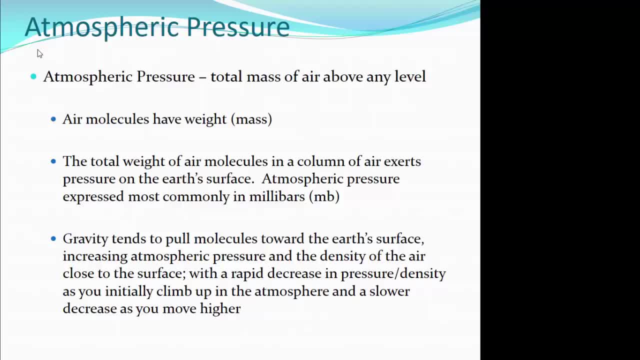 So the density, The density of the air and the pressure is higher at the surface and then goes down as you go up in the atmosphere. Oftentimes you talk about going up a mountain and we say the air is thinner up there. You've heard that, I'm sure. 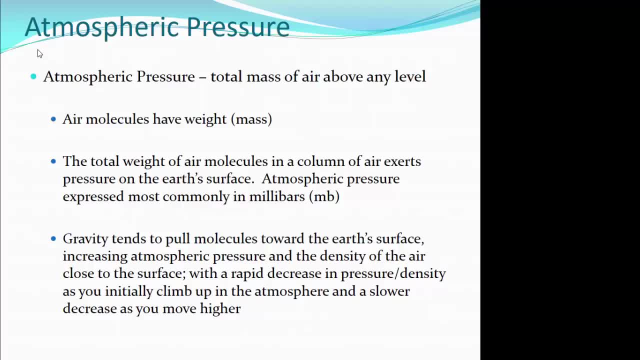 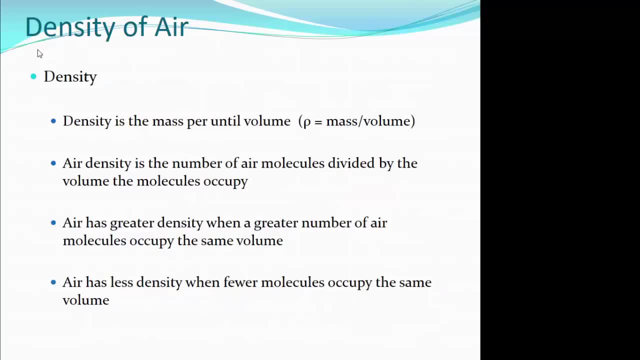 Well, that's fewer molecules as you go higher in the atmosphere. So what is the density of the atmosphere? Well, density is mass per unit volume. That little curvy P is actually the Greek symbol, rho. That's typically what's used for density. 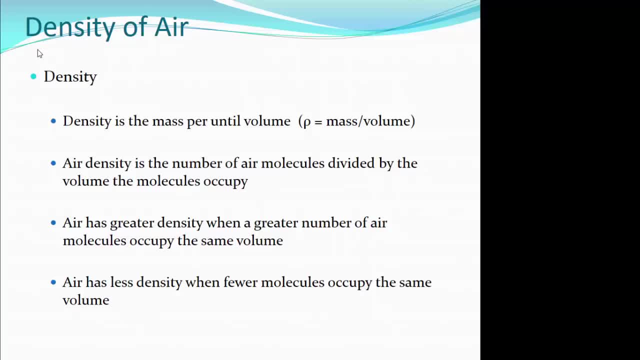 So density equals mass divided by volume. If you take a whole lot more stuff and you put it in the same volume, it's more dense. If you have less stuff and put it in the same volume, it's less dense. Take a one-inch cube of styrofoam. there's not much there. 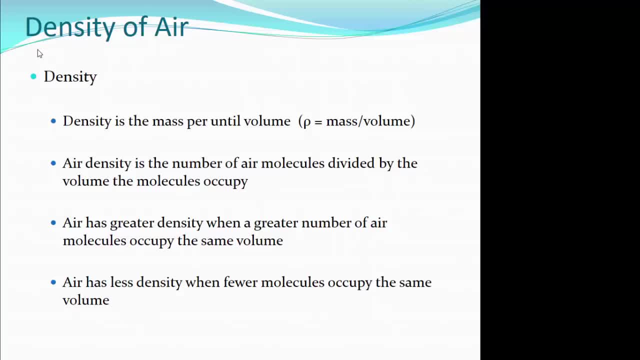 It's pretty light. Take a one-inch cube of lead and it's way, way heavier. Why? Because there's way more mass. The molecules of lead are closely packed together. The molecules of styrofoam are loosely packed together, So less mass in the styrofoam. it weighs less. 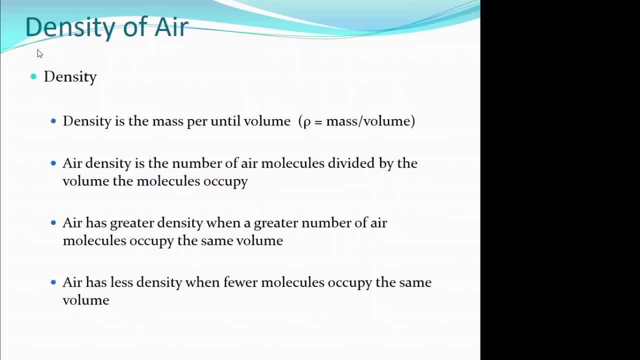 It has less density. The same volume of lead has way more density. Air density is the number of air molecules divided by the volume the molecules occupy. Air has greater density when there's a greater number of air molecules occupying the same volume. Air has less density when there are few molecules occupying the same volume. 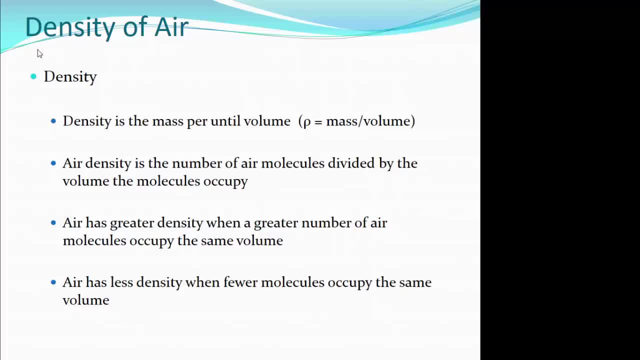 Air has less density. higher in the atmosphere The air is thinner. up there, Air has much greater density. It's closer to the surface, where there are more air molecules and the air is more dense. Now we will look at the structure of the atmosphere based on density and pressure. 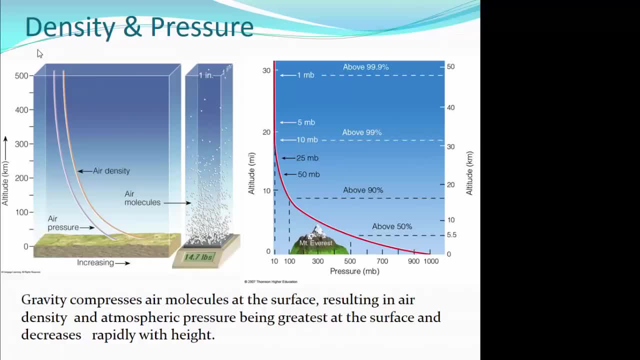 The density of the air and the pressure of the air at different levels. And we have two different pictures: the one on the left, the one on the right. On the left, the red line being air pressure, the blue line being air density. 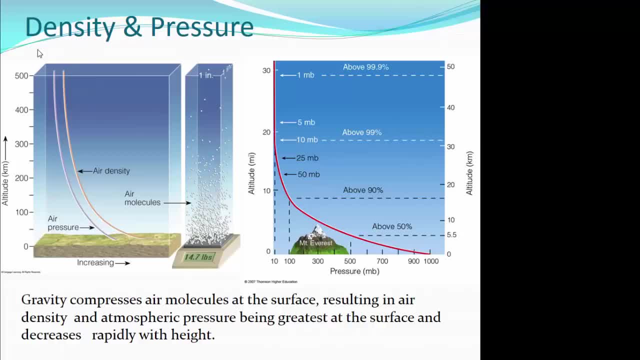 And you can see that at the surface, because on our y-axis it goes from zero to 500, that's kilometers, And on our x-axis it goes from a small amount to a high amount And in that left hand, the 80% of the picture. your air pressure and air density are high. 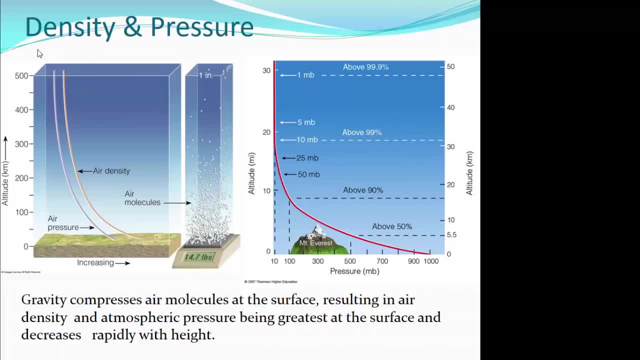 at the surface. They decrease rapidly with height initially, and then their decrease slows down as they go up in the atmosphere, And that's presented to you graphically on the right side of that picture. You can see the atmosphere there, with the air molecules being pointed out. 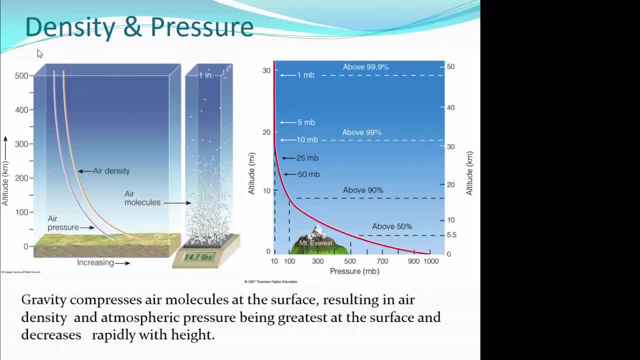 And if there are 100 air molecules there, then you know that 78 of those are nitrogen and about 20% are nitrogen, 21 of them are oxygen. So we have all these air molecules And because of gravity, most of the air molecules are pulled and they gather at the surface. 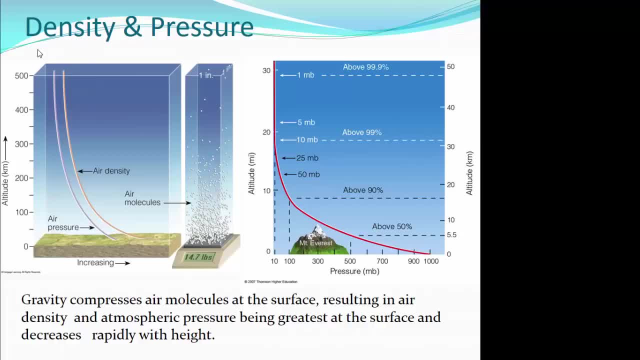 And that's why you have higher air pressure and higher air density at the surface, And both decrease with height: rapidly at first and then less rapidly as you go up in height. And again look at where we have the arrow pointing from air molecules. 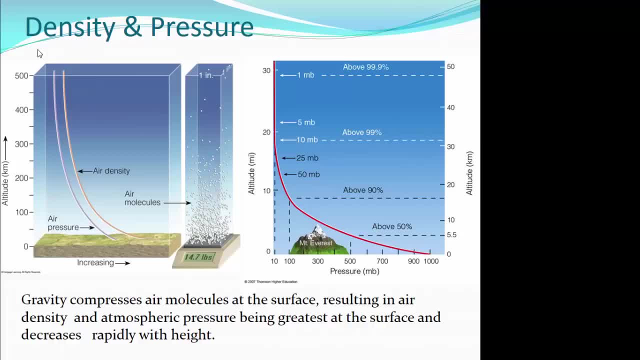 That is why we say the air is thinner up there. As you go up in the atmosphere, there are literally fewer air molecules. There are literally fewer air molecules to breathe or to take in or to use. and that accounts for going up the side of a mountain. 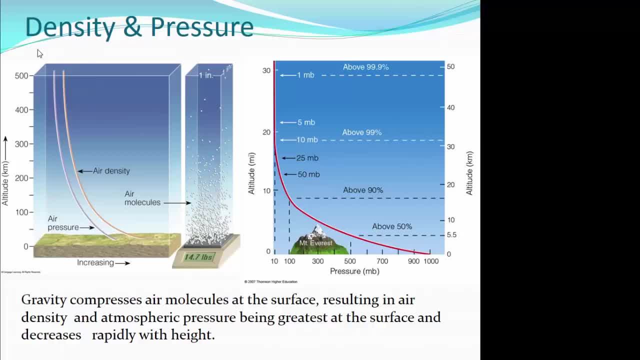 And, by the way, on the right-hand side picture you can see the mountain. And again, that X axis is from low pressure to high pressure, 1,000 millibars, That's the number we're going to use for surface pressure, generally, about 1,000 millibars. 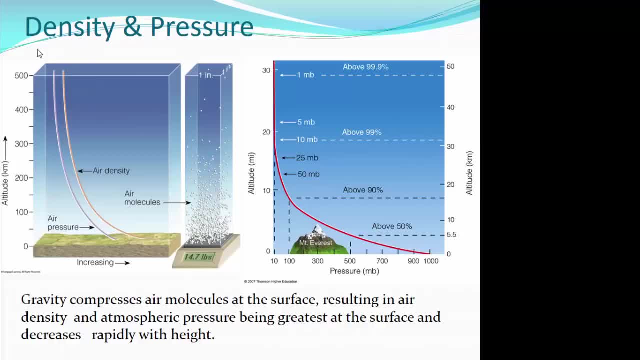 And then a zero being there all the way at the Y axis. And the Y axis again is altitude: kilometers on the right-hand side, miles on the left-hand side, And if you go up Mount Everest, just about at the summit of Mount Everest, a full 50%. 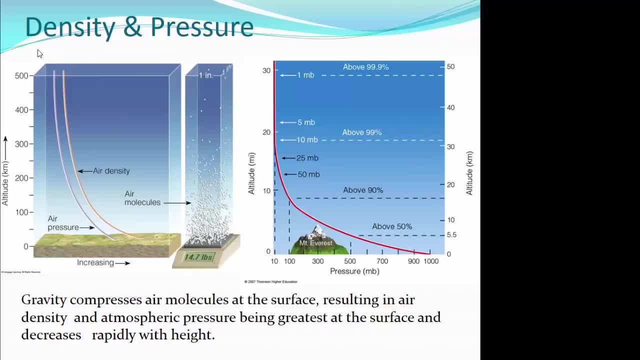 of the air molecules in the atmosphere are below that level, And you can see how that plays out in that right-hand graph. And then, as you go further up in the atmosphere, you get up to just below 10 miles and 90%. 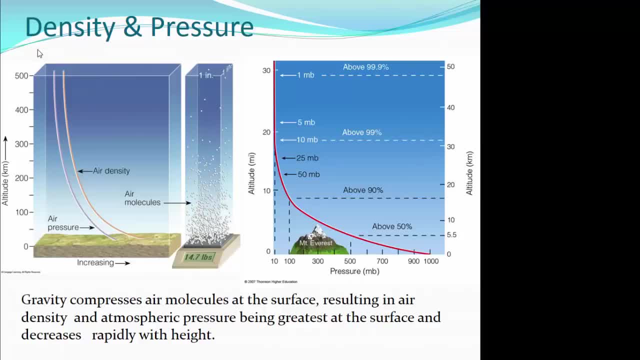 of the atmosphere is below that location, And then you get up to just below 20 miles and 99% of the atmosphere is below that, So the air is thinner up there. If you are standing at the base of Mount Everest at sea level, atmospheric pressure is about: 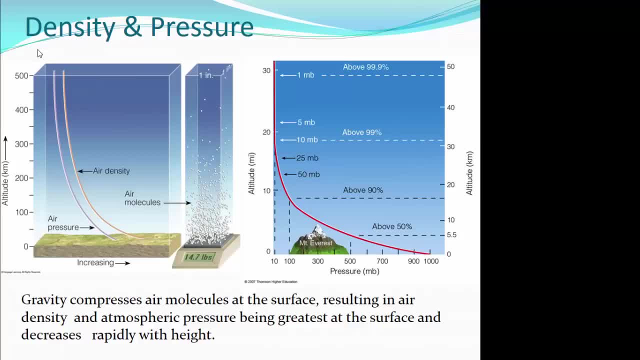 1,000 millibars. If you get to the very top of Mount Everest, what's above you there? How many molecules are above you there? At the very top of Mount Everest, atmospheric pressure may be about 300 millibars. 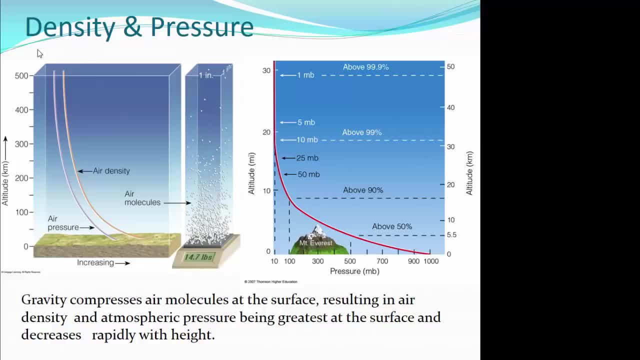 It goes down rapidly with height. If you are about 18,, 19 miles up in the atmosphere, atmospheric pressure may be 100 millibars, And the same thing happens with density. The air is very dense at the surface. We can breathe in. 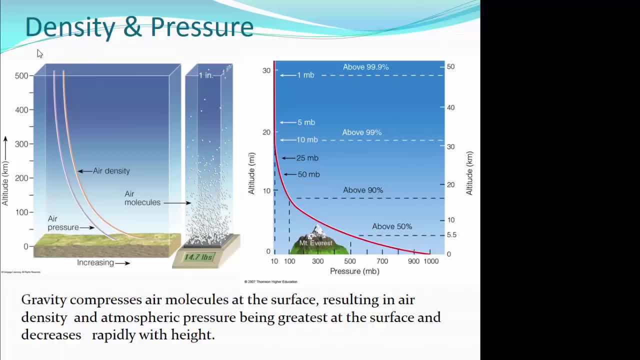 It's easy to breathe. As you go up Mount Everest, it gets harder and harder to breathe And the air density becomes much lower. The air is thinner up there. Gravity compresses air molecules at the surface, resulting in air density and atmospheric pressure. 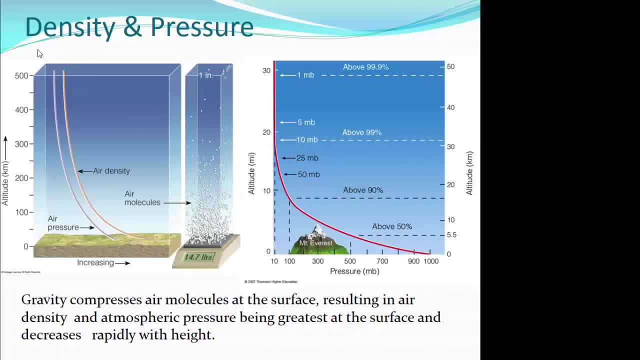 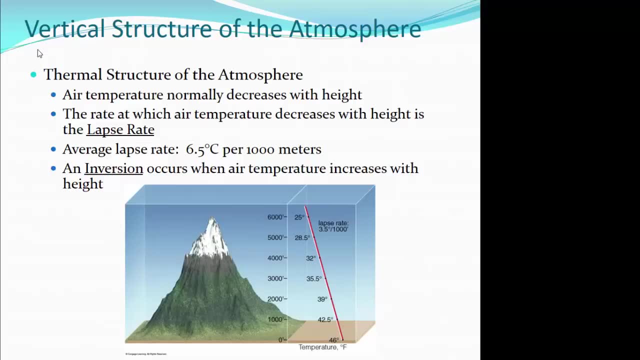 being greatest at the surface and decreasing rapidly with height. There's also a thermal structure to the atmosphere. When you go up a mountainside, does it get warmer? No, it gets colder. The higher you go in the atmosphere, it gets colder. 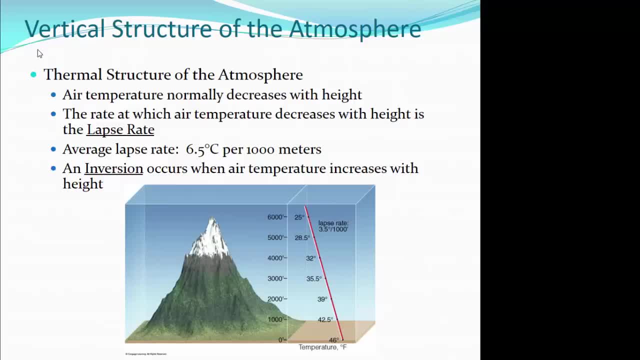 The thermal structure of the atmosphere. air temperature normally decreases the height, Not always, not absolutely, but normally decreases with height. The rate at which air temperature decreases in height is called the lapse rate. The rate at which air temperature decreases in height is called the lapse rate. 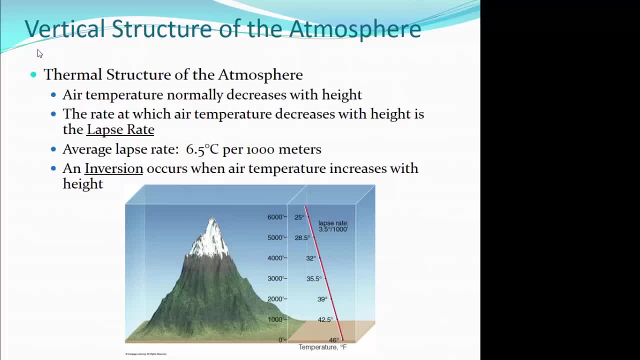 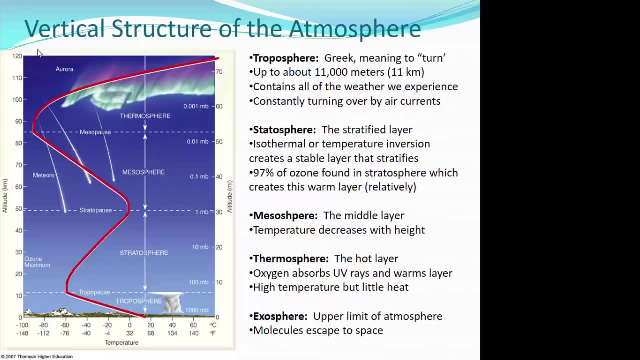 The average lapse rate is about six and a half centimeters per 1,000 meters. An inversion occurs when air temperature increases in height. We can classify the vertical structure of the atmosphere Based on temperature Many times in this class. I will tell you that science is all about classification. 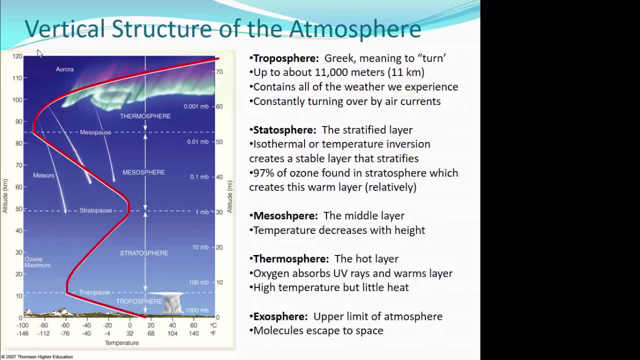 Scientists classify things. If you have a shell scientist and he gathers 10,000 shells at the seashore, he may take all the pink shells and put them in one pile, and all the fan-shaped shells and put them in another pile, and all the cone-shaped shells and put them in a third pile. 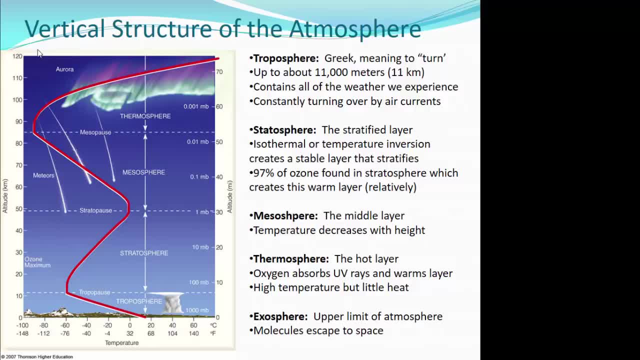 And then that scientist will then classify each shell based on the pile it's in. So scientists classify- And here we're going to classify The different levels of the atmosphere based on the thermal structure, the vertical thermal structure of the atmosphere. So let's start at the surface, where we are and know, the very first layer of the atmosphere. 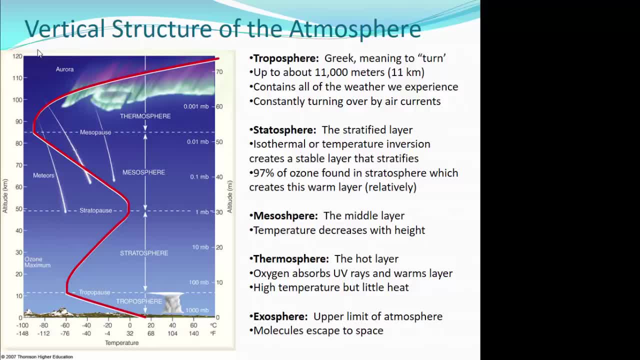 based on thermal structure, is known as the troposphere. Now, tropo is a word that means to turn, Because in the troposphere the air is constantly turning. There is upward vertical motion- air is going up- and there is downward vertical motion. 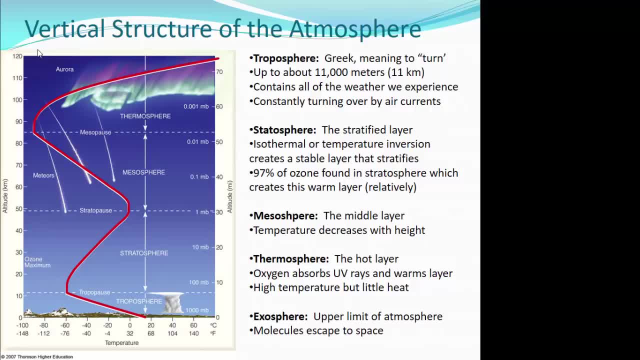 air is going down. Air can rise off the surface or sink down to the surface, And that constant turning creates the troposphere. Nearly all of the weather that we experience, virtually all, occurs in the troposphere. At the top of the troposphere, the dashed line is the tropopause. 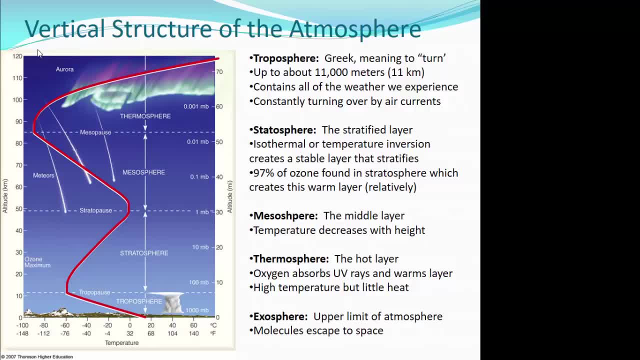 That separates the troposphere from the next layer of the atmosphere, the stratosphere. And then of course you see, above the stratosphere is the stratosphere, The stratopause, And then above the mesosphere, the mesopause. 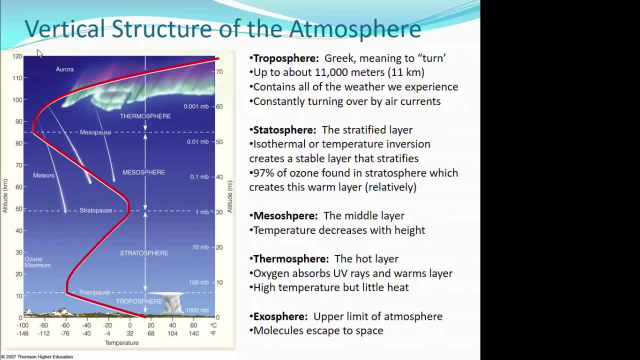 Let's talk about why there's these thermal structures or thermal layers In the lowest layers of the atmosphere. the environmental lapse rate, or the rate at which temperature decreases with height in the environment, is again about 6.5 degrees Celsius per thousand. 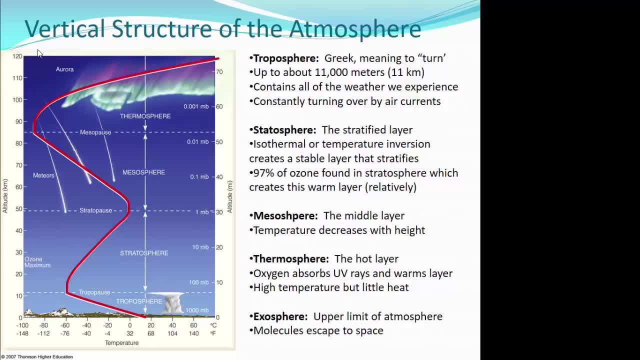 meters And you can see our red line. We start there at the surface at about 59 to 60 degrees Fahrenheit And that line then goes down. It decreases with height until you get up to the tropopause. It's a pretty steady, constant decrease. 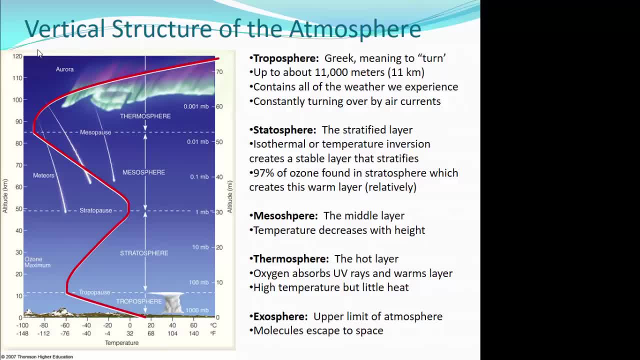 Now in the real atmosphere, there may be fluctuations in that temperature drop and there may even be very small layers in which temperature increases for a distance with height, those small inversions, But generally it is a decrease all the way up to the tropopause. 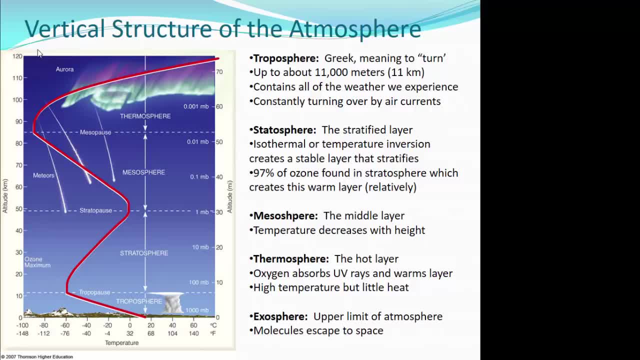 So the troposphere up to about 11,000 meters contains all the weather that we experience, constantly turned over by air. It turns and the air temperature is falling At the tropopause above for a few miles. actually, the temperature remains the same. 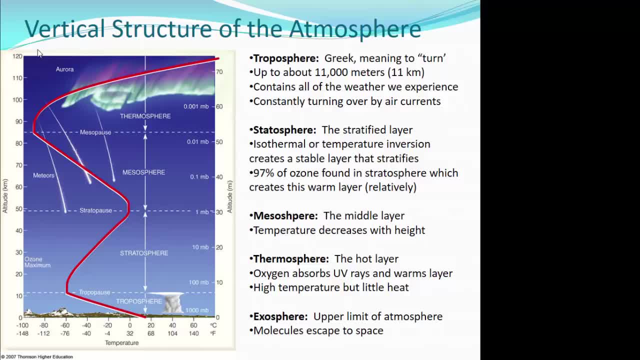 We refer to that as isothermal, It remains the same. And then comes the first big inversion where air temperature increases with height. Now I'm not telling you that it's warm up there. Those air temperatures are still 20,, 30,, 60 degrees below zero Celsius and up to 75 degrees. 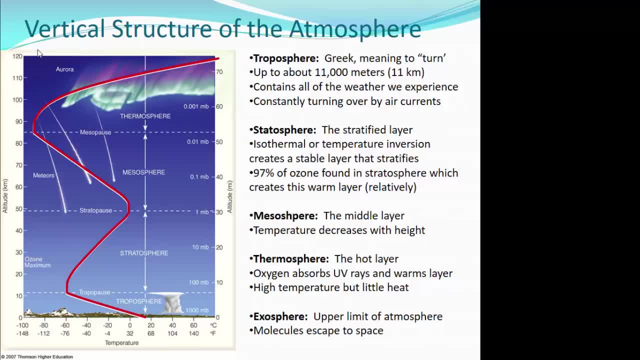 below zero Fahrenheit. So it's very, very cold, But the temperature actually increases. The temperature actually increases with height And you can see on the left between 20 and 30 kilometers up the ozone maximum And that's why temperature increases with height in the stratosphere. 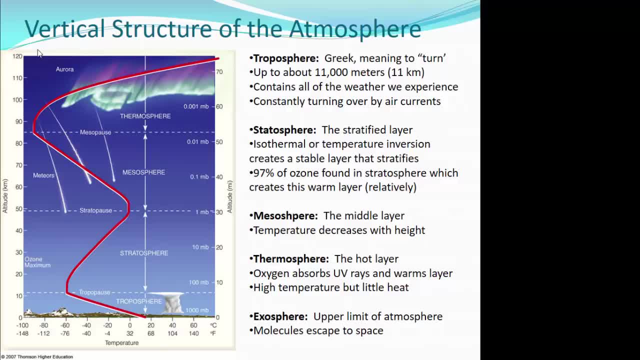 That's where all the ozone is, And ozone is an excellent greenhouse gas. It absorbs the infrared radiation. It absorbs all the radiation- the sun, the ultraviolet specifically- And those molecules of ozone begin to move very quickly and therefore they warm up. 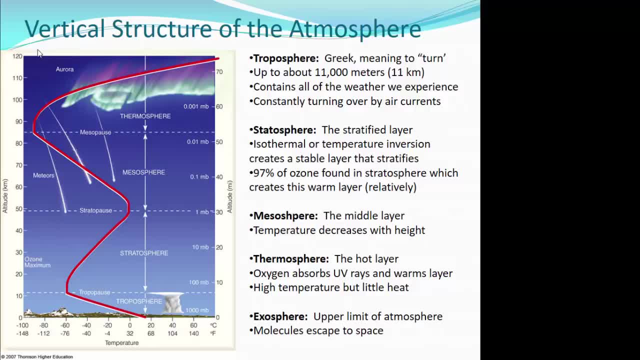 creating the stratosphere. The air actually gets warmer as you go up. Because air is warm as you go up, It is stratified. Strato is a term that means layered. The stratosphere is the stratified layer, Isothermal or an inversion. it creates a stable layer that stratifies. 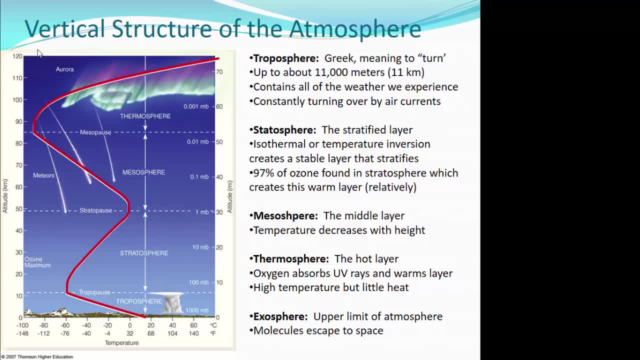 97% of the ozone is found in the stratosphere, creating this warm layer. So why is air getting warmer as you go up? Why is that a stable atmosphere? Why does that stratify the atmosphere? Well, warm air rises right. 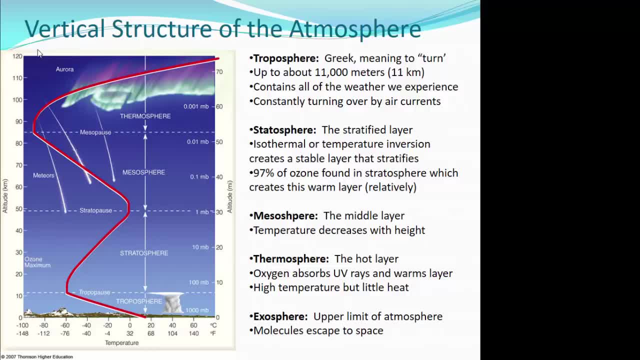 Hot air Balloons go up, Warm air rises. If the air above you is even warmer, then that balloon will not go up. It'll actually sink back down, And that's the stable aspect of the stratosphere. But the stratosphere is the mesosphere. 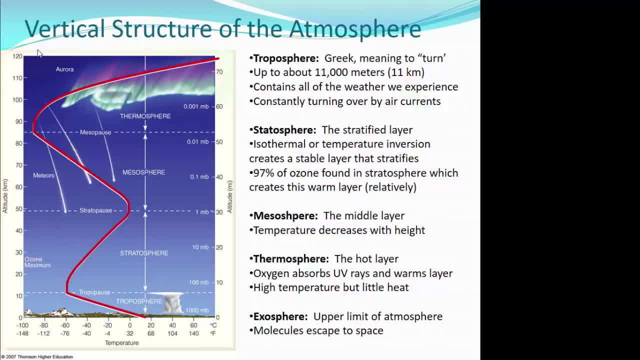 The middle layer temperature again decreases with height And then in the exothermosphere into the exosphere you see a rapid increase with height. But again there are so few molecules of air, so few molecules of nitrogen or oxygen that 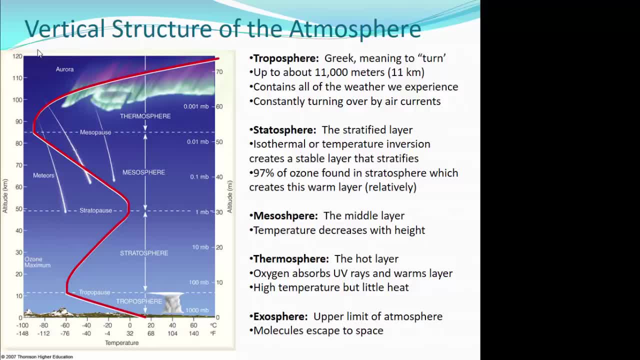 even though they may be moving very, very quickly because they're being agitated or excited by the interplay Incoming solar radiation, There's so few molecules that you actually can't feel that heat. Yes, the individual molecules may have high speed and therefore high temperature, but 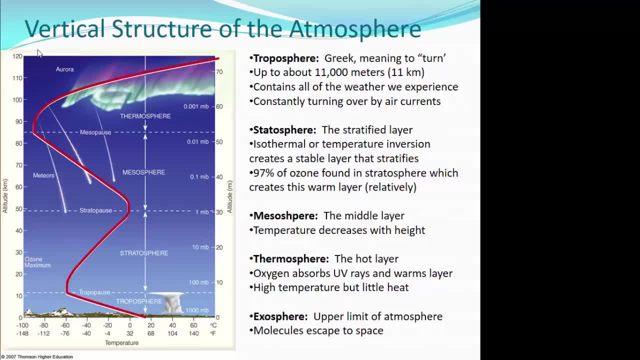 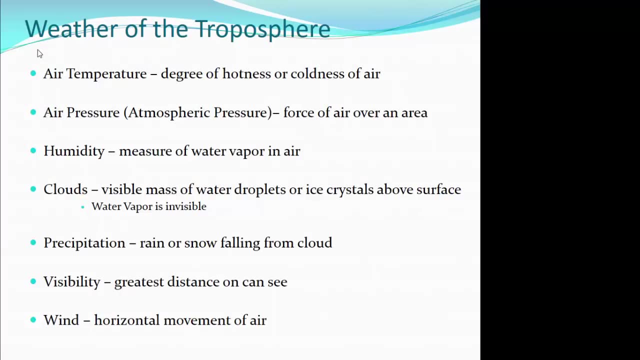 there are so few molecules you can't actually feel that heat. So that high temperature of the thermo and exosphere is a bit understood. You can't actually feel the heat up there. The molecules are just moving that quickly. So what type of weather is in the troposphere? 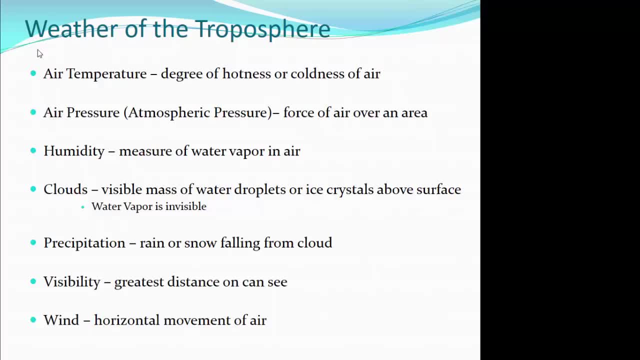 Air temperature, Air pressure, Clouds, Precipitation, Visibility And wind- Things you've mostly all heard of And you already know what they are: The temperature, The degree of hotness or coldness of the air. The air pressure or atmospheric pressure. 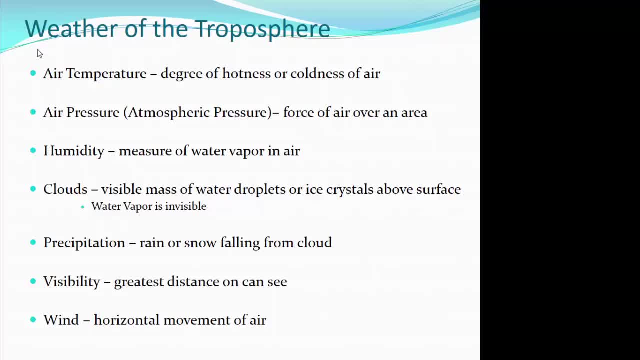 Force of air over a given area, Humidity, The measure of water vapor in the air Clouds, Visible mass of water droplets. Now get this. Water vapor is invisible. If it's vapor, it's invisible. Look around the room that you're in right now. 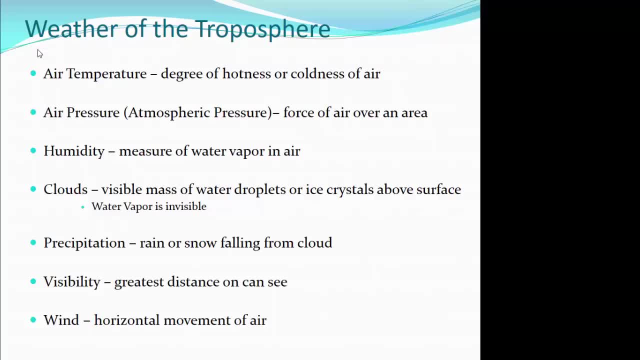 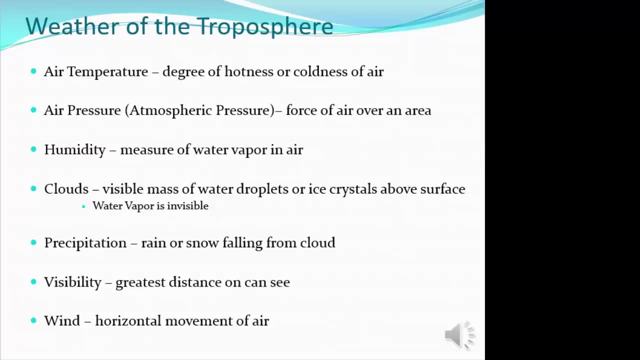 There's humidity in that room, Maybe not much. There's water vapor in that room. You just can't see it. Water vapor is invisible. Water vapor is basically individual water molecules floating around in the atmosphere. When molecules condense into droplets- water droplets- they become cloud droplets. 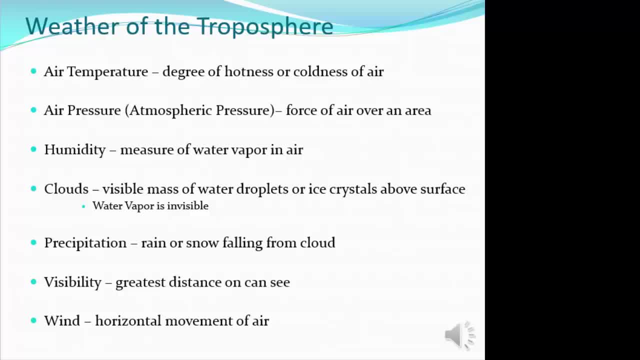 And a mass of water droplets is a cloud. Those water vapor molecules can also freeze into ice crystals and show up as clouds. If enough ice crystals form together and grow large enough, it can follow snow. If enough water droplets grow together and become water droplets, they become clouds. 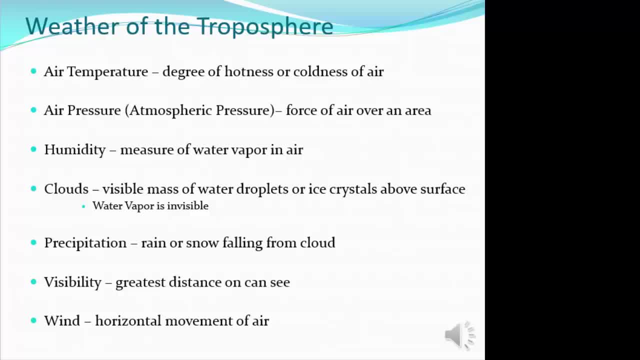 If enough water droplets form together and grow large enough, it can follow snow. The visibility of the pressure is, of course, the distance. Once you scale it down you can see how different it is from what you traditionally check in quáters or a. 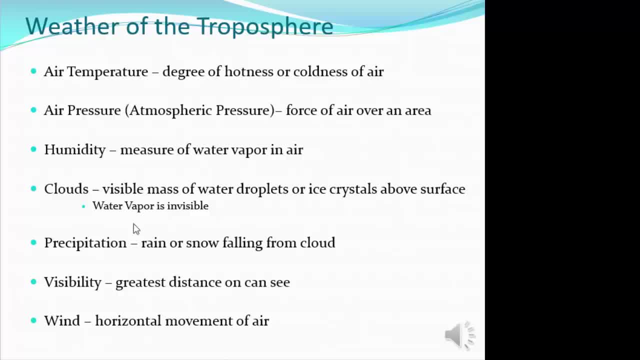 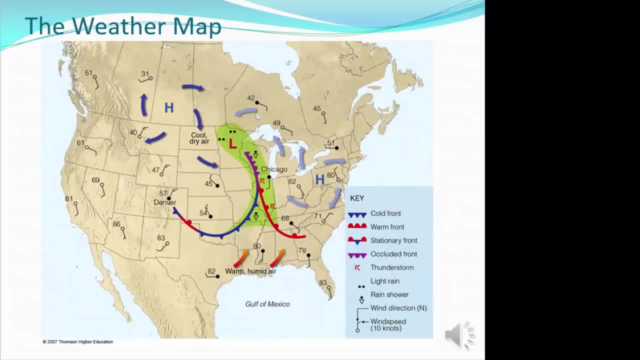 pen, It's an influence on kayaks or it can also be influenced by flow. Can you see that This is a synoptic surface weather map? Surface map, of course, because it's showing the features of the surface, Synoptic meaning at the same time. 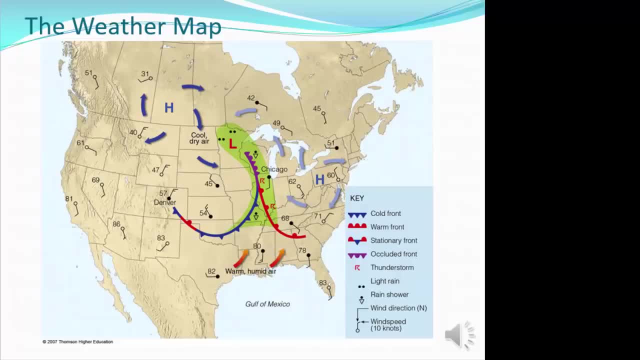 telling us that we know that the temperature in British Columbia is 51 degrees, while the temperature in Lake Okeechobee is 83. at the same time, The other features you see are the high pressure centers, with winds blowing clockwise and outward from the highs. 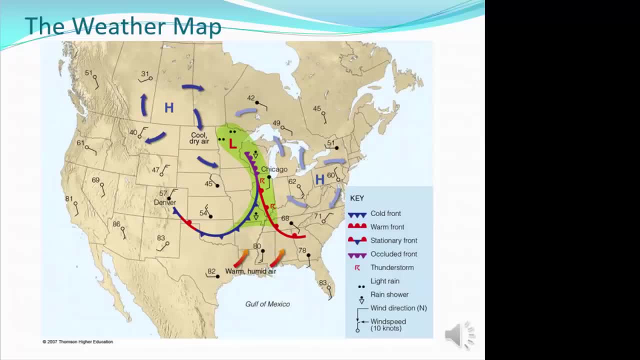 the low pressure centers, with winds blowing counterclockwise and inward into the lows, and, of course, the fronts that are associated with that area of low pressure. Why are there fronts? Fronts are simply the leading edge of a certain type of air mass replacing another air mass. 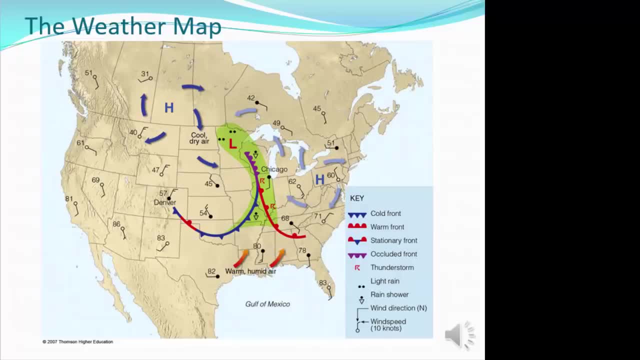 In the case of the cold front, that is cold air replacing warm and humid air. In the case of the warm front, it is warm and humid air replacing cold air, With this area of low pressure and the counterclockwise flow around it. 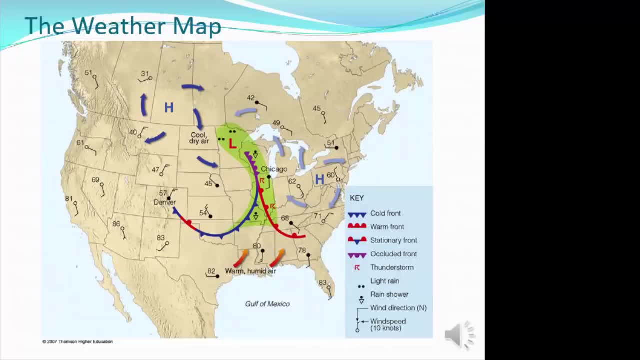 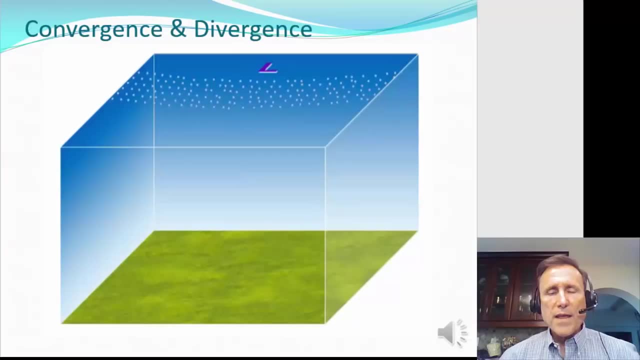 it's bringing cold, dry air out of Canada south and creating that cold front- the leading edge of the cold air- and warm, moist air off the Gulf of Mexico to the North, creating that warm front. All right, that's going to pretty much bring. 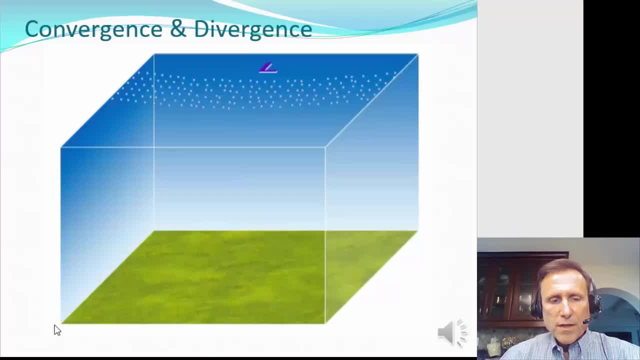 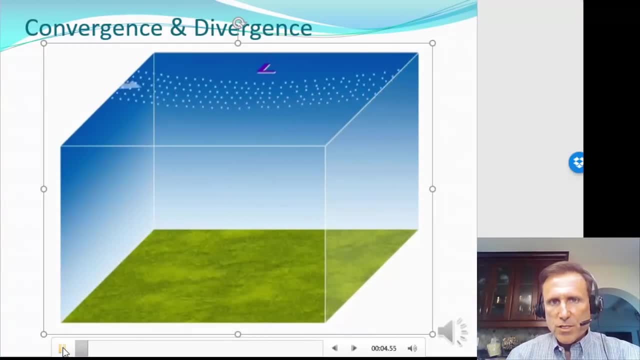 this part of chapter one to an end. I want to leave you with an interesting illustration or a little video here showing that the surface features I just talked about are connected to the upper level features And what you're looking at at the top of this cube. 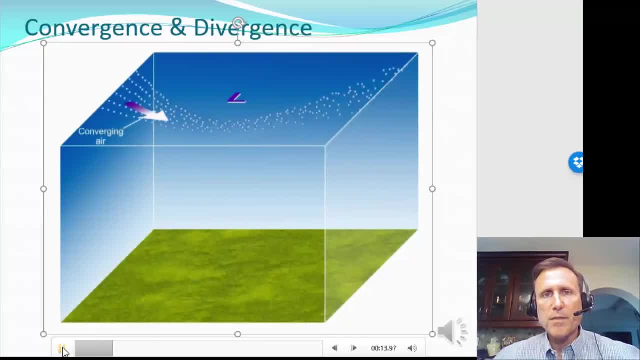 are the upper level winds- Winds blowing at 15,, 20,, 25,000 feet up in the atmosphere, And where those winds go around around what would be an upper level low. as the winds move into that upper level low, they converge.